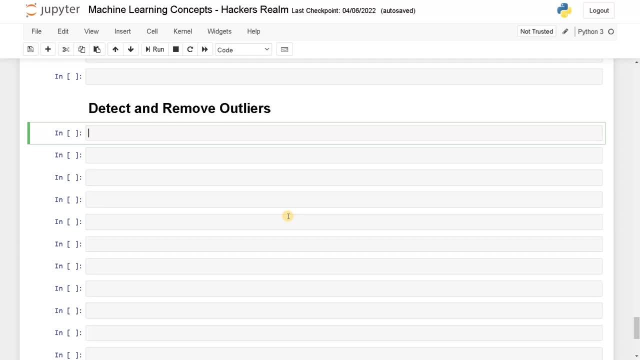 some pre-processing and improving the quality of data. Now let's get into it. First I'm gonna use Wine Quality Dataset. for this, I have already loaded the dataset. Now I'm going to use one particular column called Residual Sugar, So I will also get the details. 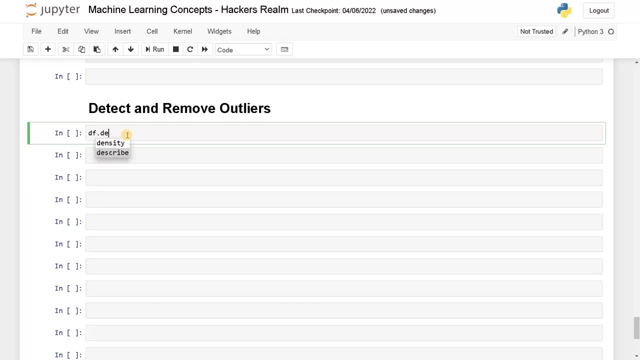 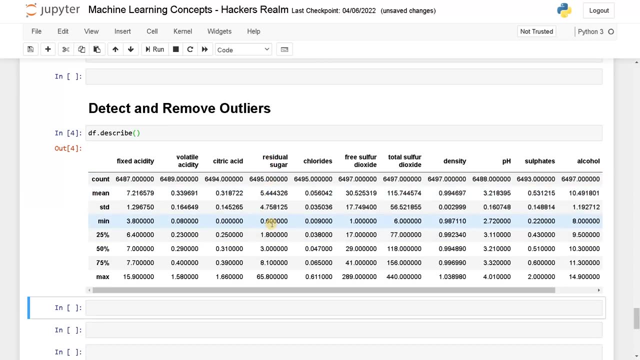 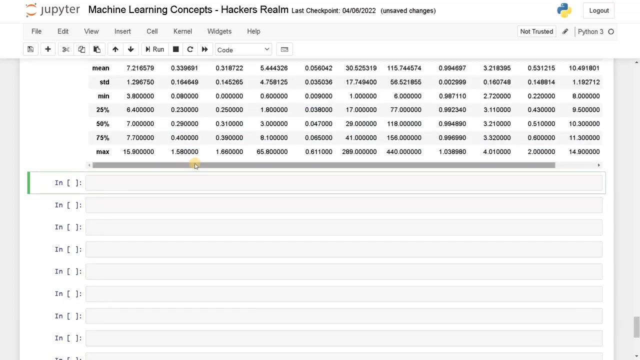 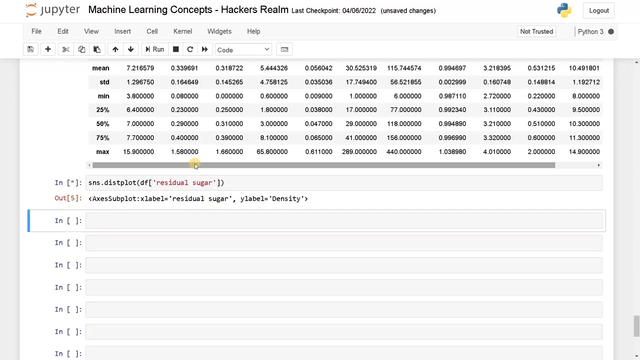 df of describe of the whole data. So I'm gonna use this residual sugar. So the minimum value is around 0.6 and the maximum value is around 65. Now let's plot the data. snsdescribe This plot df of residual sugar. run this Now you can see there is definitely an outlier. 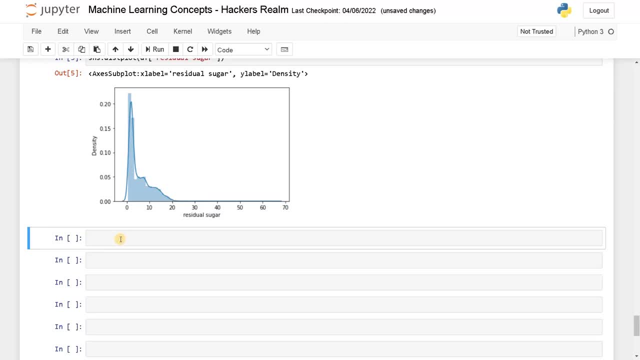 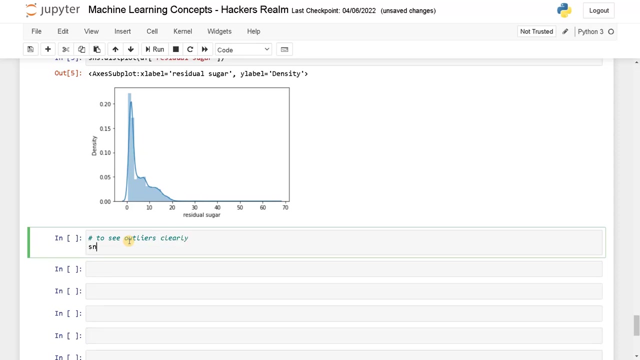 because this data is completely right-squared. Now, in order to see the outliers very clearly, we can use BoxCut to see outliers clearly. snsbox-plot df of residual sugar sleep outlined at the전�ering side of the content. 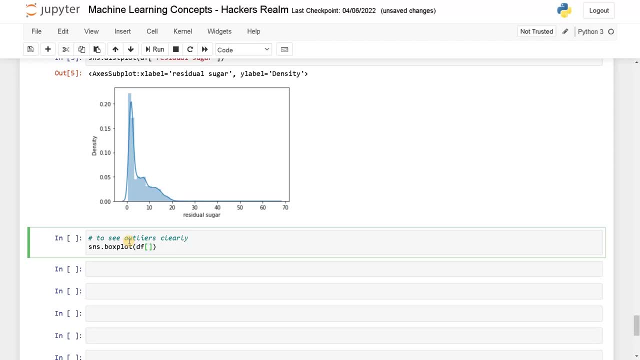 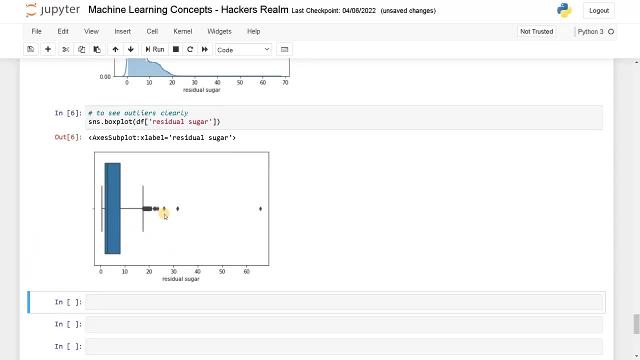 edges of the data is here: Confirm Can萝 ハ- residual sugars. now you can clearly see the interquartile range is in the range of like 0 to 18 or something, and remaining rest of the things are considered as outliers. only few of the samples are outliers, so what you can do, 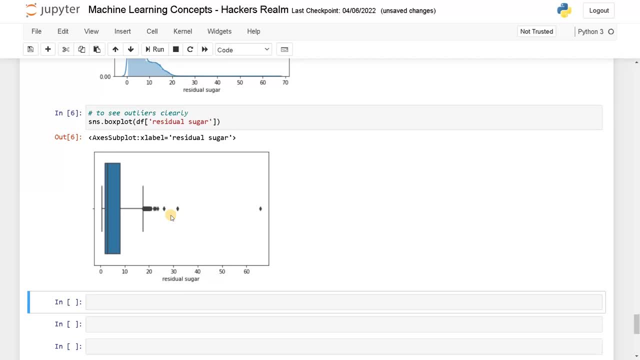 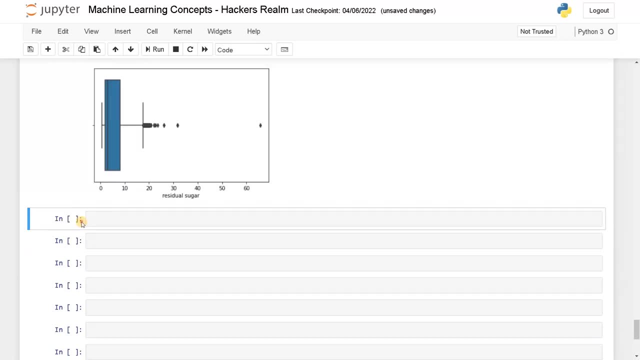 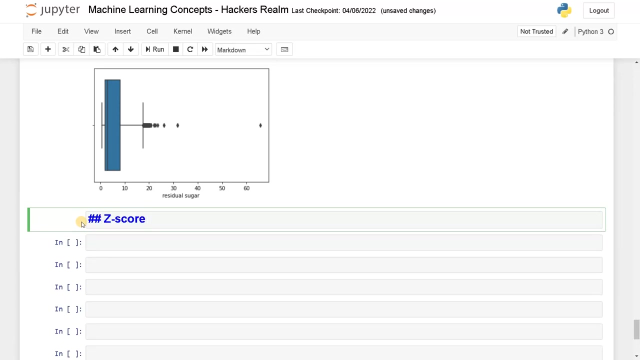 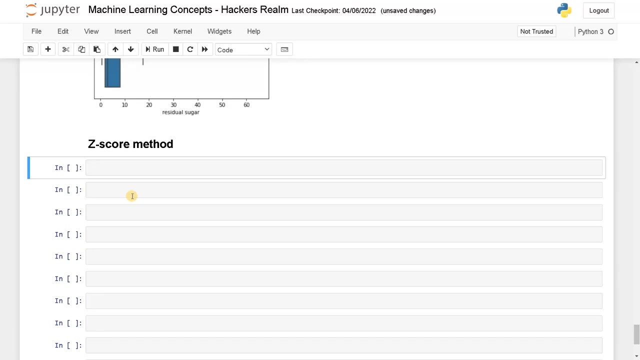 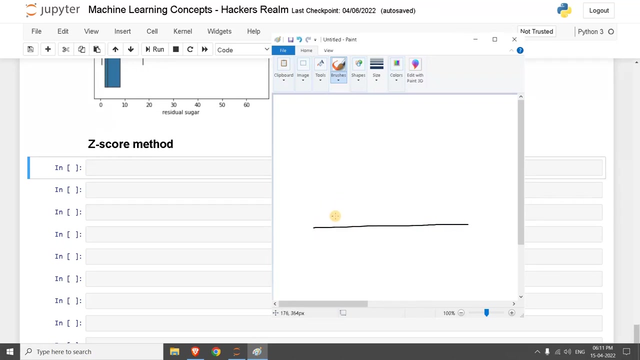 is, we can use different methods in order to remove this outliers. first method: we are going to use this z-score treatment. so this is the first one z-score method. so first I will explain how this method works. so let's open up a paint. now, here you can see. I'll just draw a distribution of a normal distribution. 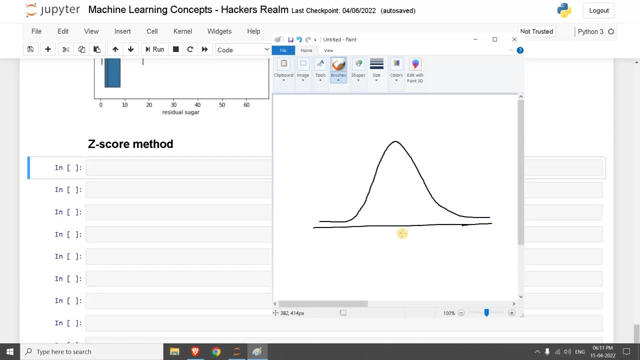 like this. so this will be considered as like mean and that will be zero and we will be having standard deviation. i will say one standard deviation to standard deviation and three standard deviation. so all these things are standard deviation. forgive my diagram. so this will be mean and this will be standard deviation. what So this is our XML, This is the table, And now let us every train links and hackers everywhere. So let us use the whole data set to become our SDK своих digital dense. 你我们在这里介入. Claus can do multiple. 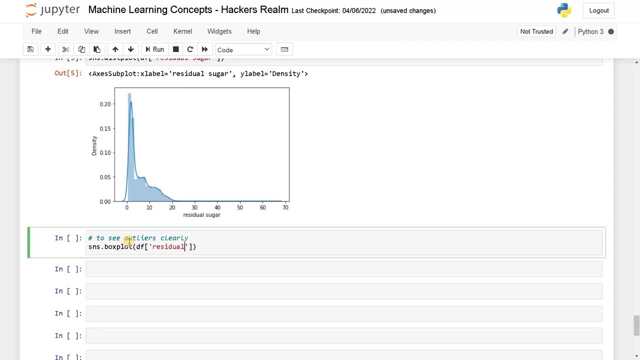 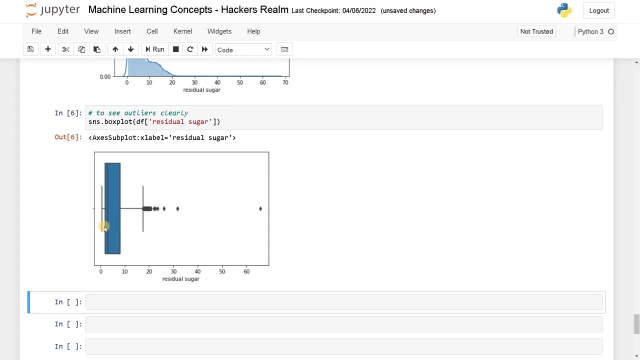 specialized instance медial propor werden. Let us say we want classes using open mestad dob statt of a vf of residual sugar. run this residual sugars- now you can clearly see the interquartile range is in the range of like 0 to 18 or something, and remaining rest of the things are considered as outliers. only few of 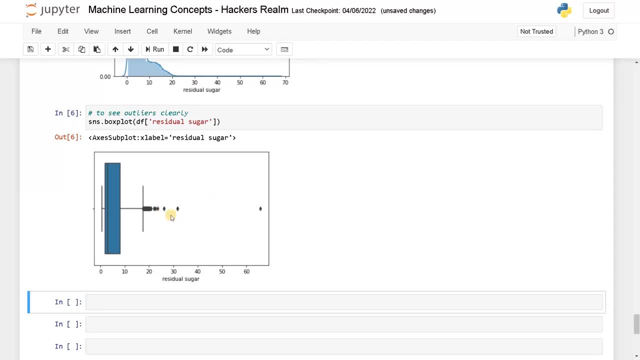 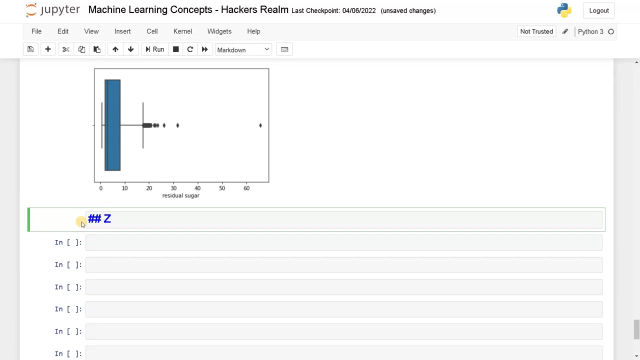 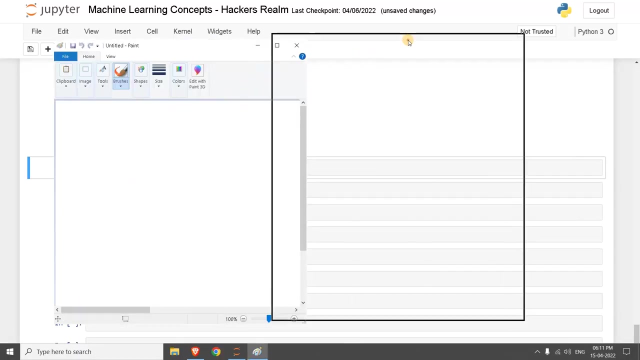 the samples are outliers. so what you can do is we can use different methods in order to remove this outliers. first method: we are going to use this Z score, our treatment. so this is the first one Z score method. so first I will explain how this method works. so let's open up a paint now here. 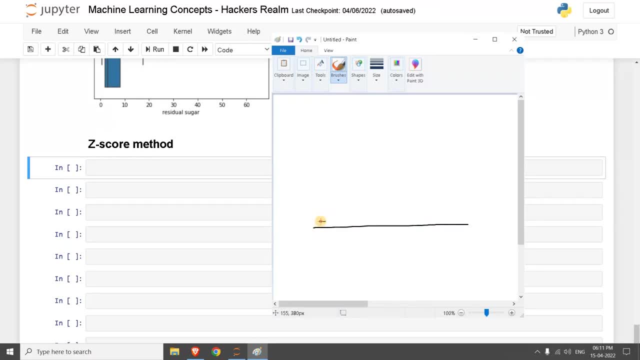 you can see, I'll just draw a distribution of a normal distribution line like this. so this will be considered as like mean and that will be zero and uh, we will be having standard deviation. i will say, uh, one standard deviation, two standard deviation and three standard. 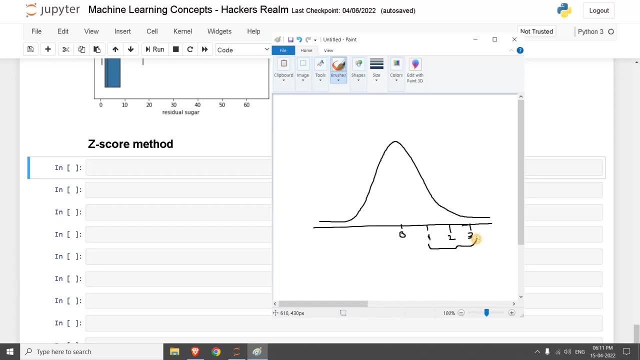 uh deviation. so all these things are uh, standard deviation. forgive my diagram, so this will be mean and this will be standard deviation. what we will be doing is we will be taking only uh, the values, that is, in, uh, in the range of three standard 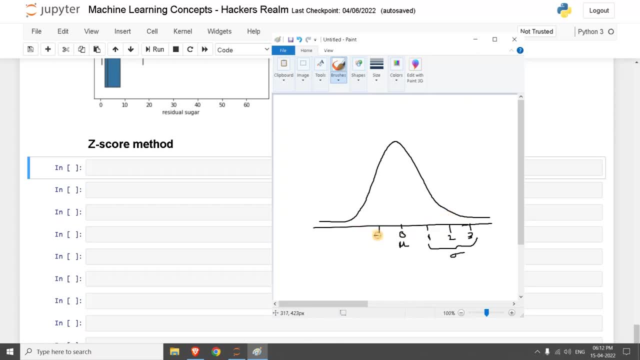 deviation. so i will take uh plus or minus three standard deviation, so so i'm gonna take until these values. so this will uh be considered as a lower limit and this will be considered as a higher limit or upper limit. so i will call it as. 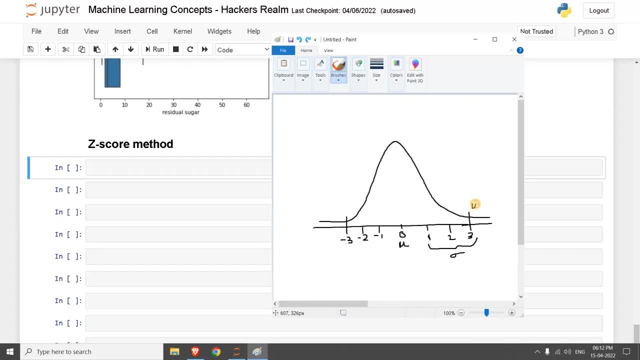 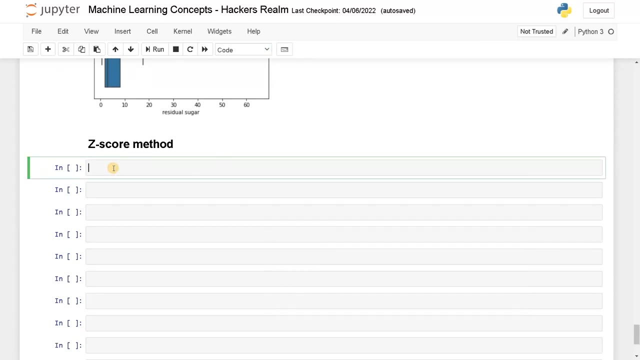 uh, upper limit and this will be lower limit. okay, both are l okay. so this is the first method we are going to use. so we already plotted the distribution. now i will say upper limit. upper limit equals df of residual sugar, dot mean minus, sorry, plus three, multiplies df of 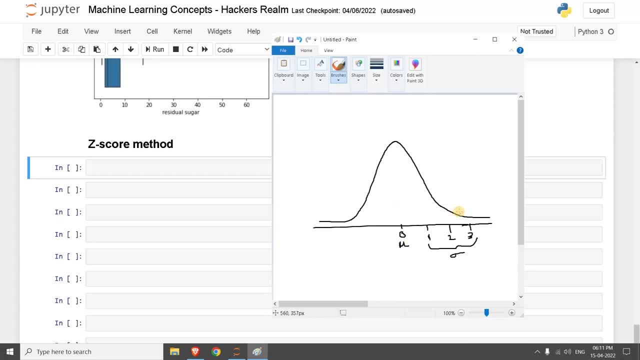 we'll be doing is: so we'll be taking only are the values, that is, in the range of three standard deviation. so I will take a plus or minus three standard deviation. so so I'm going to take until these values. so this will be considered as a lower limit and this will be considered as a higher limit, or 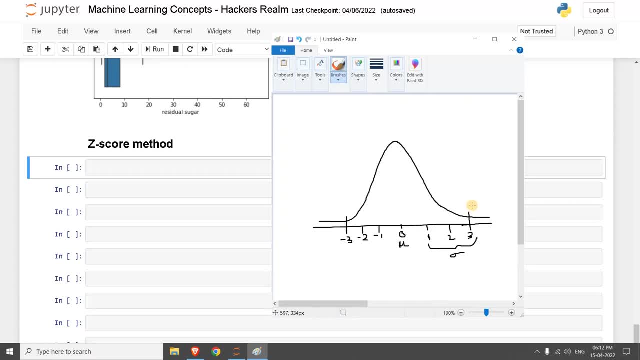 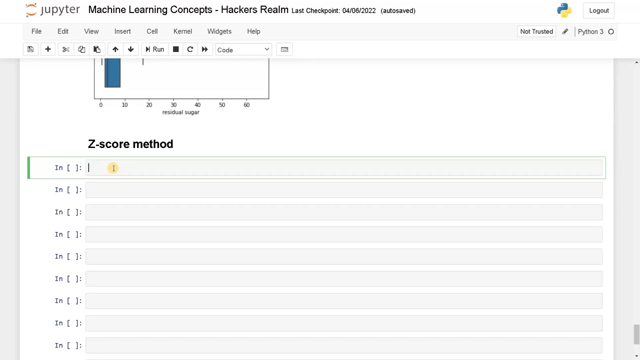 upper limit. so I will call it as upper limit and this will be lower limit. both are l okay. so this is the first method we are going to use. so we already plotted the distribution. now I will say upper limit. upper limit equals D Mike D of residual sugar dot mean minus minus one k C plusама minus one k plus 10. 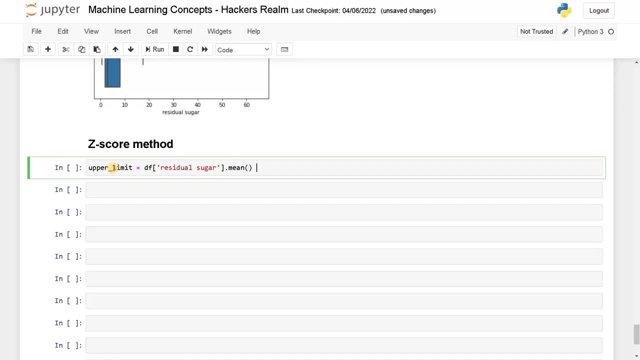 square kит 1 inclusively. well, this is an applauseek, which is: this: does a total of 128, our difference between the drugs, because we thought we were going to evaluate it, the value number. fine, just so, we have to do number which is equal to 148 if Lustran, we have 0 math. 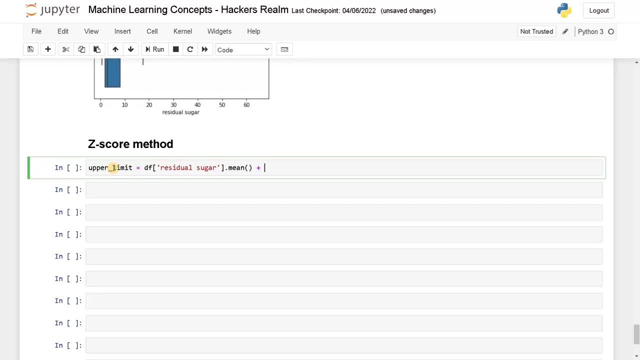 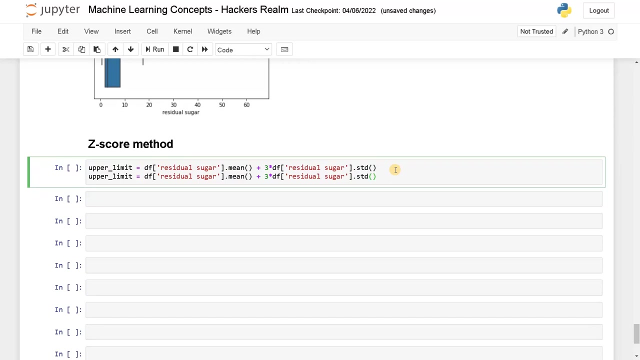 fixed and the dürfen we fixed in Q and X. but in order to solve this problem, because minus- sorry, plus 3 multiplies df of residual sugar, dot standard deviation, So this is 3 standard deviation I am getting, So similarly I am going to get the lower limit. So this: 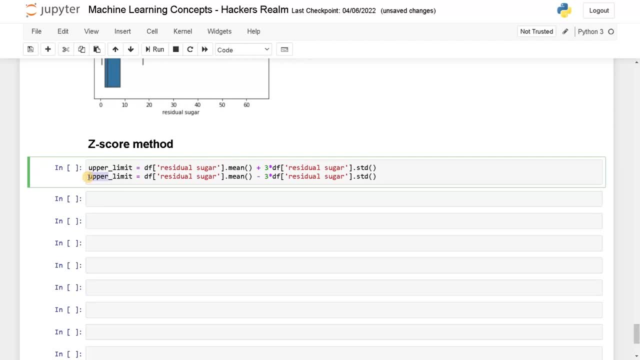 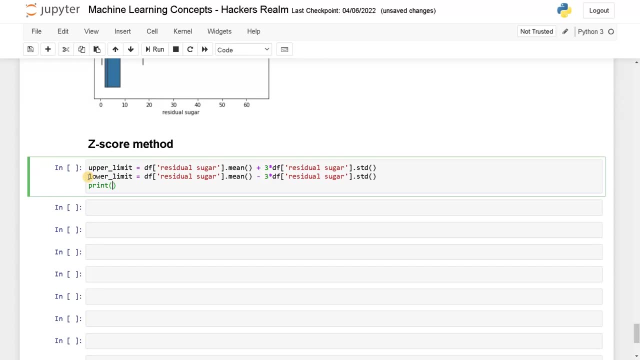 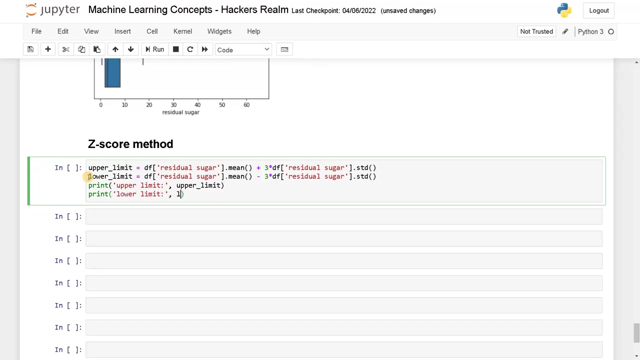 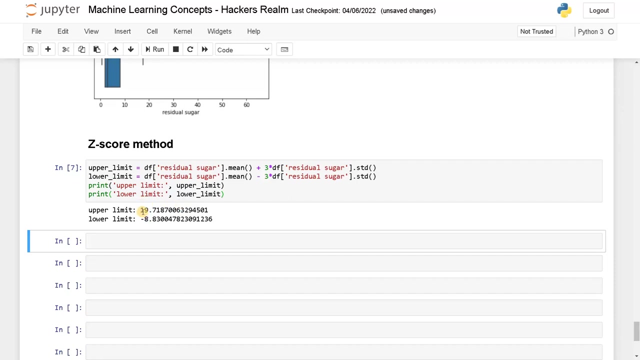 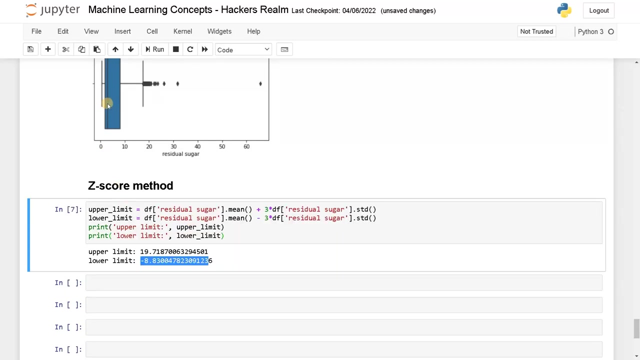 will be minus to get the lower limit. After that, let us print it So: upper limit, upper limit and lower limit. Okay, Now you can see this is the possible upper limit that we can consider and this is the possible lower limit we can consider, But the lower value is around like 0.6.. So in 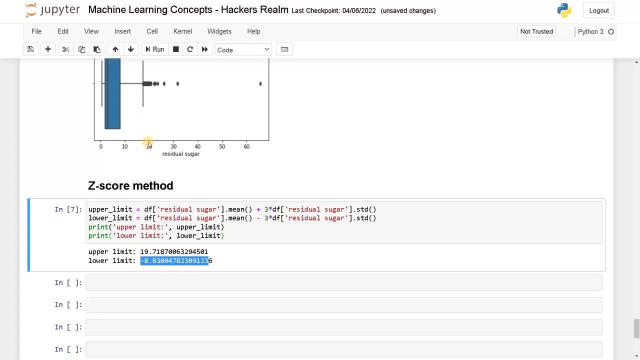 the negative side, it is not an issue, But on the upper side, we are going to consider around like 20.. So, as you can see, these are the values are considered and rest of the values will be removed. So, using this limit, first let us find the outliers, Find. 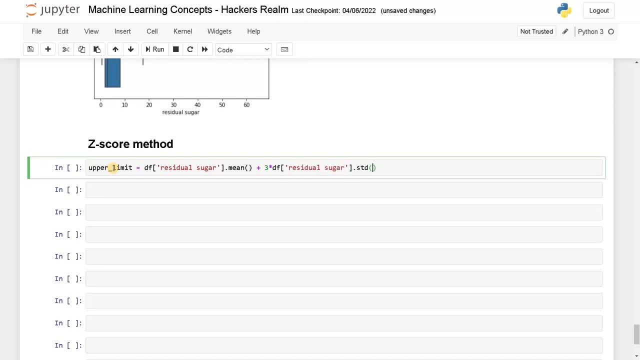 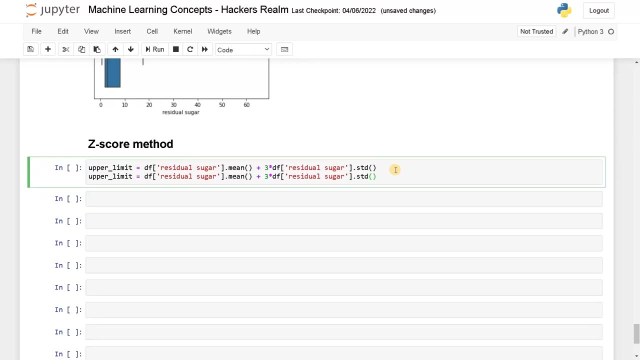 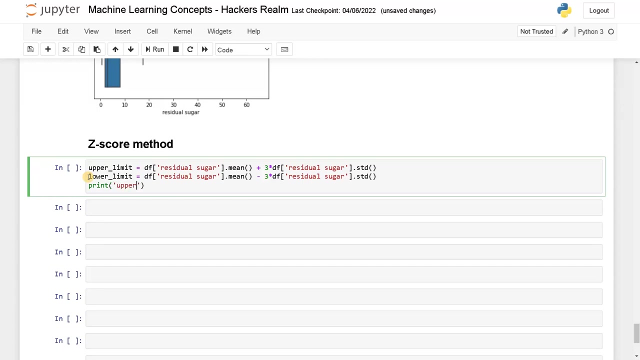 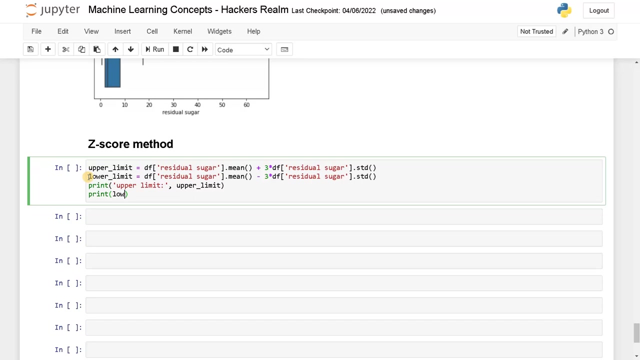 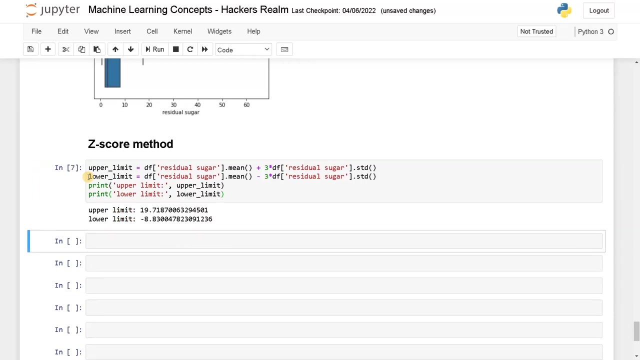 residual sugar dot standard deviation. so this is three standard deviation i'm getting. so, similarly, i'm going to get the lower limit. so this will be minus to get the lower limit. okay, after that, let's print it so: upper limit, upper limit and the lower limit, okay. 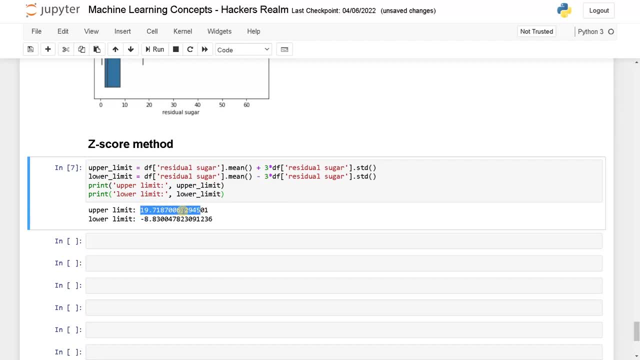 now you can see, this is the possible upper limit that we can consider and this is the possible lower limit we can make this bit now that i can see. now let me show you some combustion auto limit times. bar critical engine should be very high now the многие Lumos. 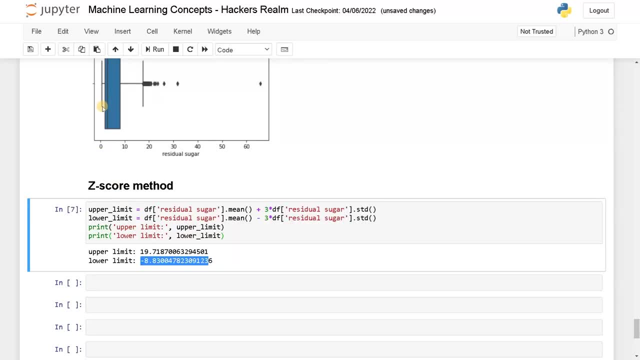 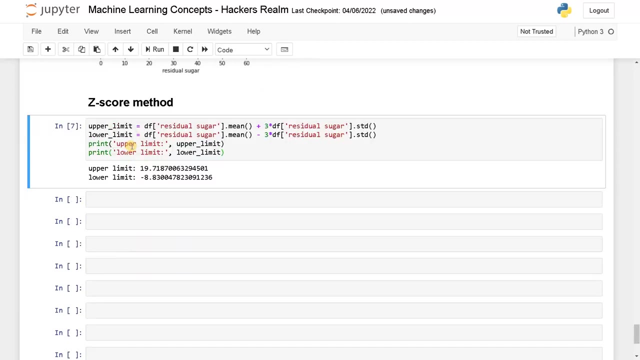 we can consider, but the lower value is around like 0.6. so in the negative side it's not an issue, but on the upper side we are going to consider around like 20. so, as you can see, these are the values are considered and rest of the values will be removed. so, using this limit first let's find. 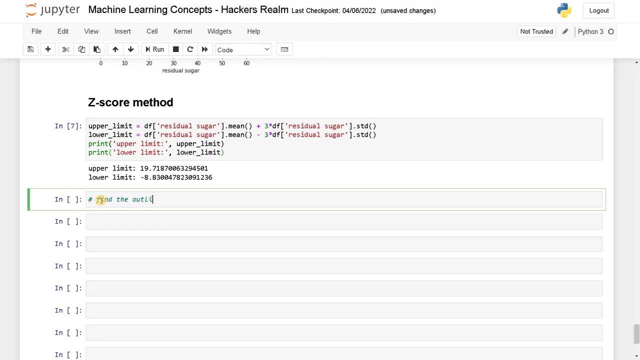 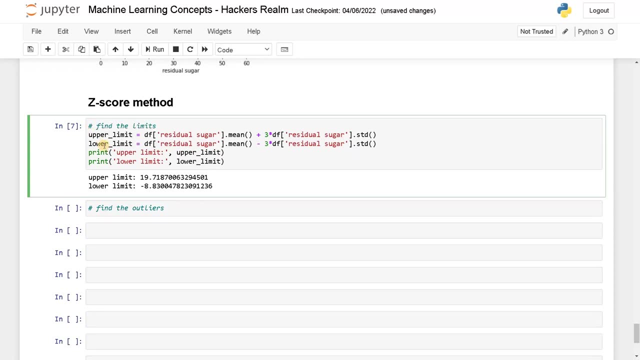 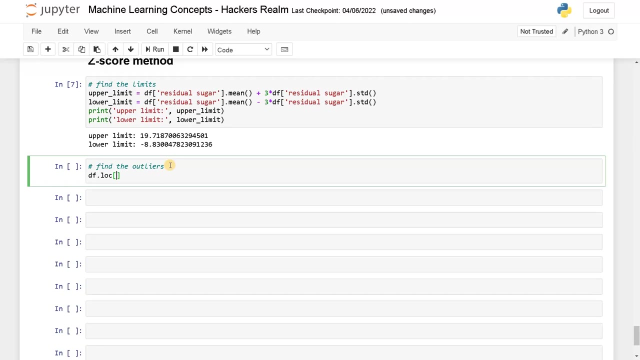 the outliers. find the outliers, and this is find the limits. so, to find the outliers, what we can do is df dot, log of df of residual sugar that is greater than upper limit, or df of residual sugar, df of residual sugar less than lower limit. okay, and from this let's display it. 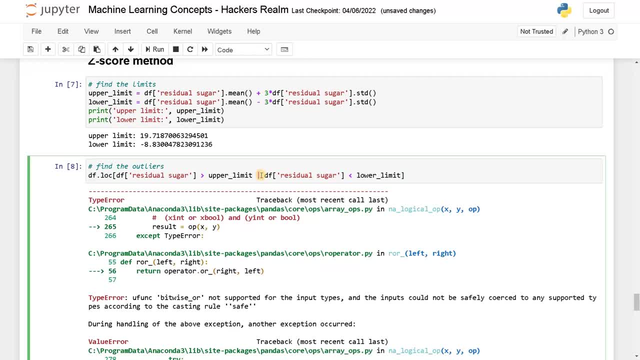 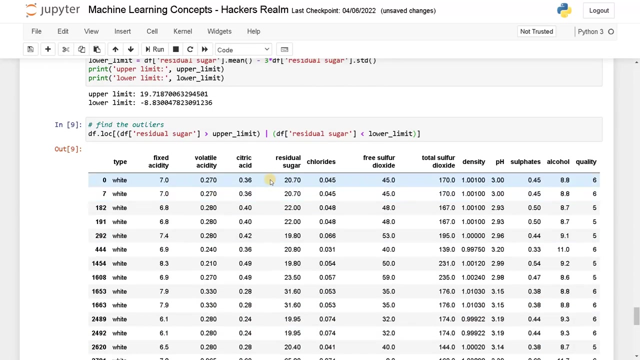 okay, i think we can use. okay, you have to do it in brackets because can lose. this will return a boolean value. if you do it as a comparison, run this now you can see: these are the outlier values. that is in the data frame. now that we find the outliers, uh, we can do two. 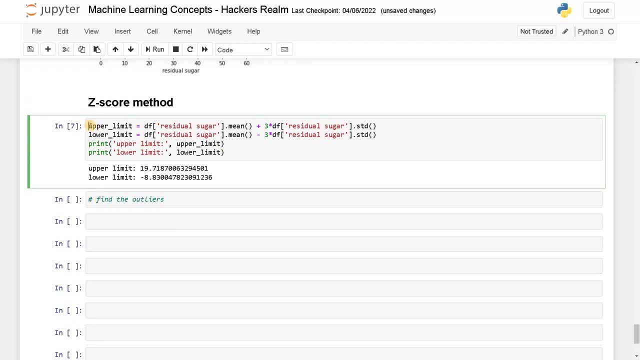 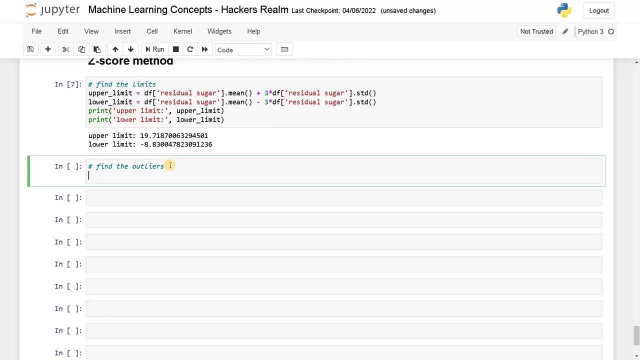 the outliers, And this is find the limits. To find the outliers, what we can do is df dot, log 0 of df of residual sugar that is greater than upper limit, or df of residual sugar greater than upper limit. Okay. 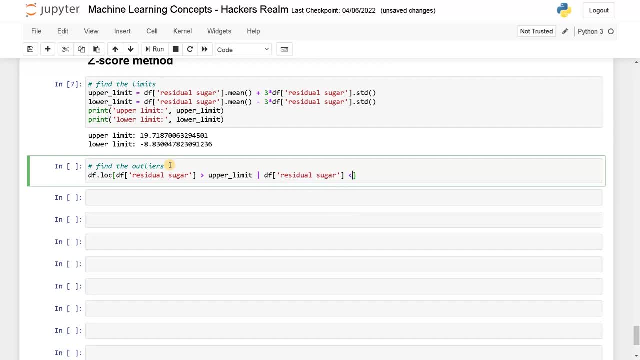 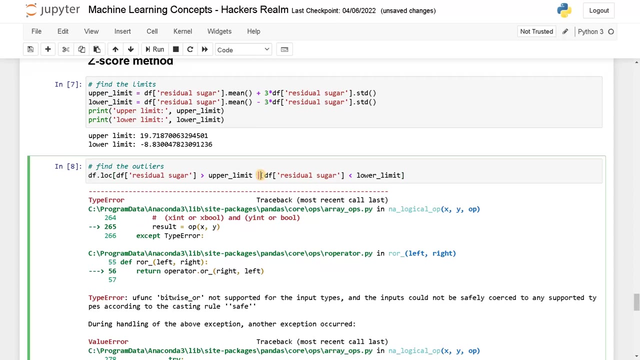 Okay, Let us now find the moreorderweis. Okay, Here we got to find F of residual sugar, So that is going to be greater than upper limit, or df of residual sugar, sugar less than lower limit, and from this let us display it. I think we can use you. 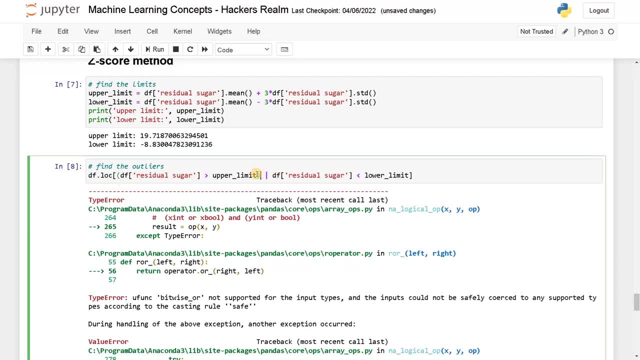 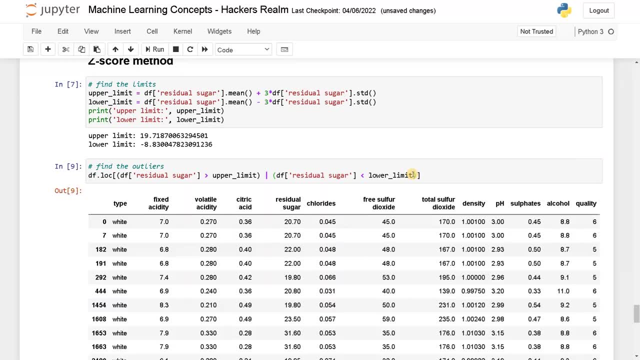 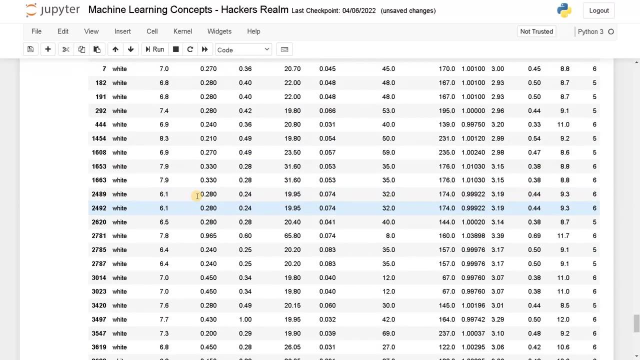 have to do it in brackets because this will return a Boolean value. if you do it as a comparison, run this now: you can see: these are the outlier values. that is, in the data frame. now that we find the outliers, we can do two things. one is trimming and another. 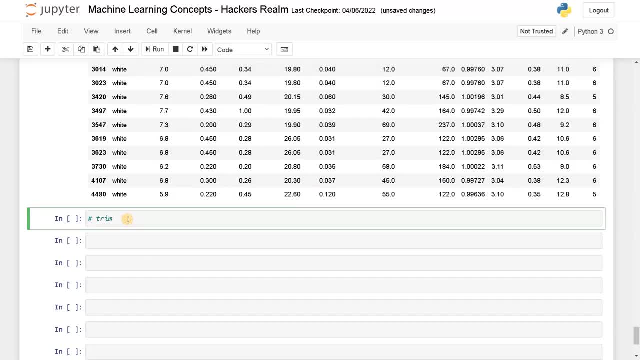 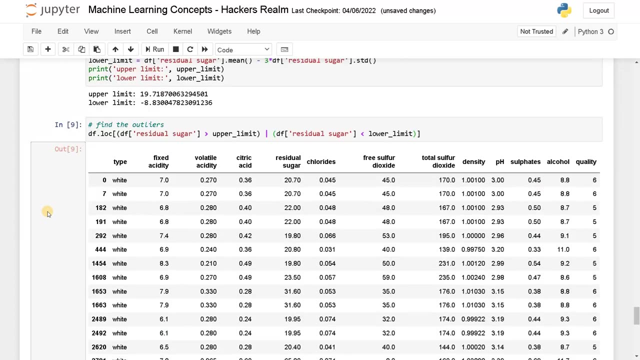 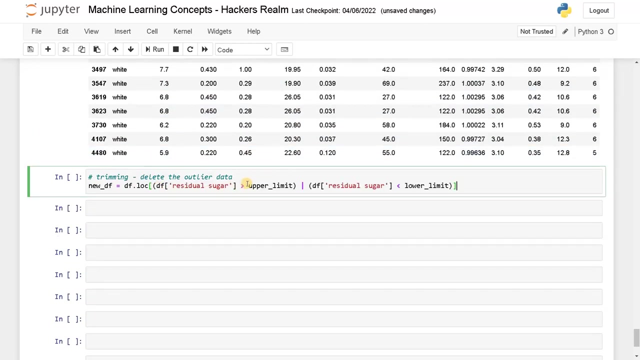 one is capping. so first we will see trimming. trimming means delete the outlier data. new df equals: again we will be doing the same condition, but instead of finding the outliers we are going to remove it. so we have to do the opposite. so I will take the values that 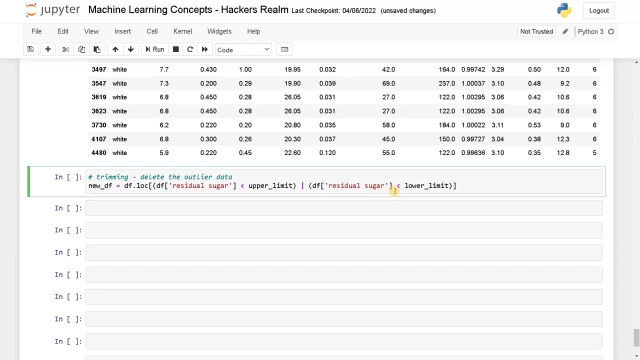 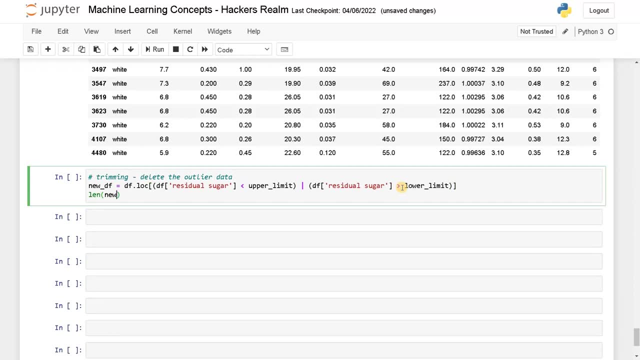 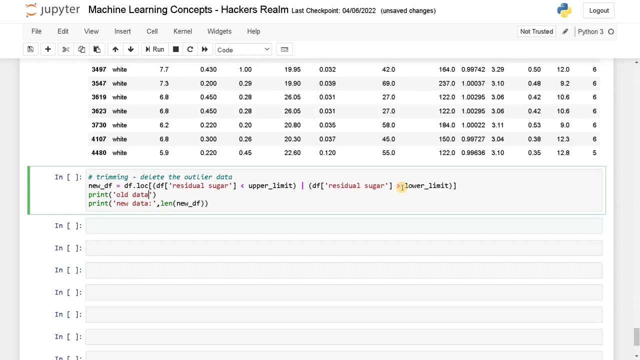 are less than the upper limit and I will take the values that is greater than the lower limit. Now I will say len of df. 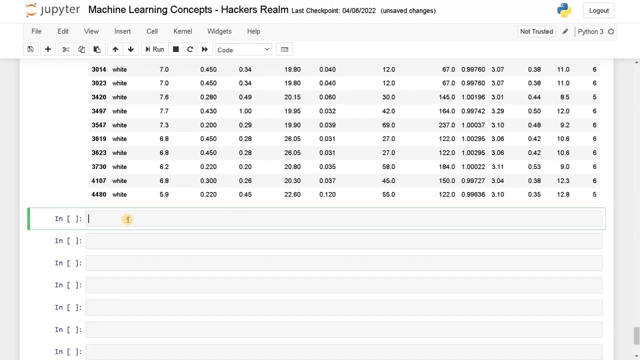 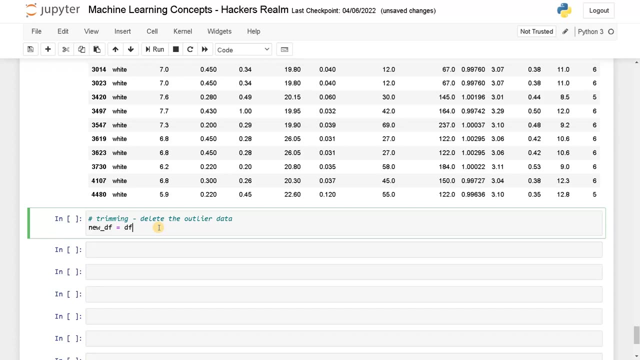 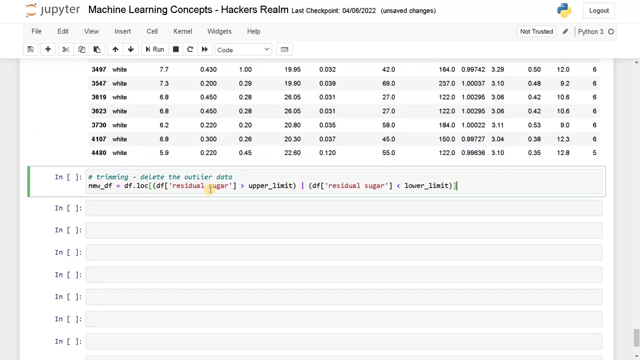 things. one is trimming and another one is capping. so first we will see trimming. trimming means delete the outlier data. new df equals. again we'll be doing the same condition, but instead of finding the outliers, we are going to remove it. so we have to do the opposite. so i will take the values that are less. 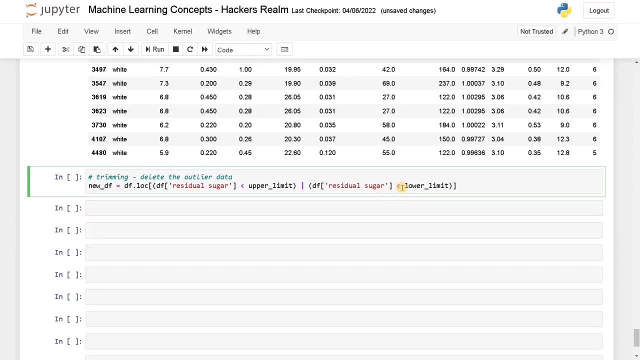 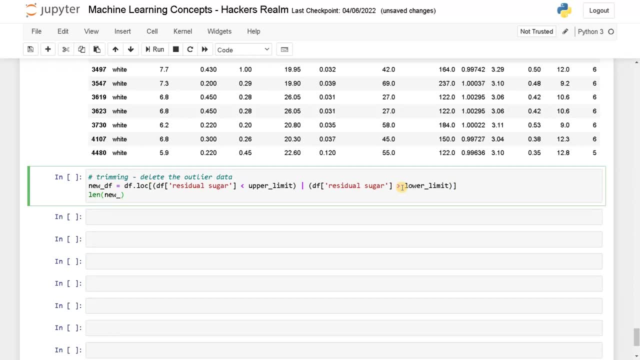 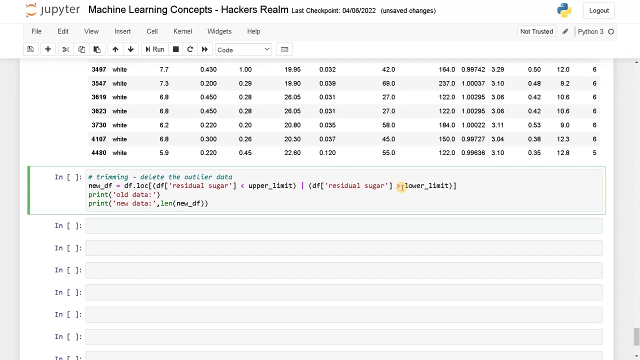 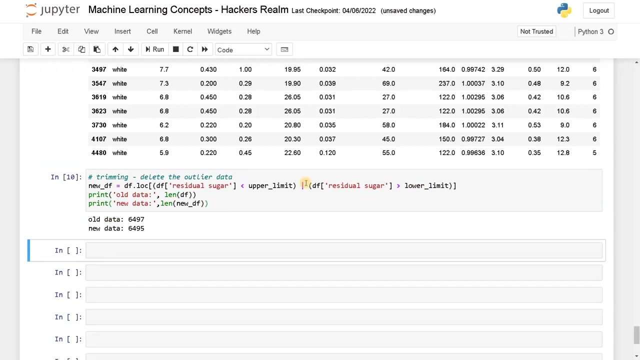 than the upper limit and i will take the values. that is greater than the lower limit. now i will say len of df. maybe we'll just print. so this will be new data, new data and another one old data. len of df. now let's run this. okay, this is, and instead of r, run this. 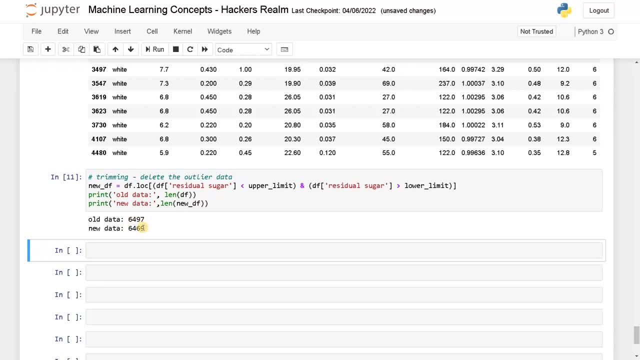 now you can see: uh, the old data length is 6497 and from that we have removed some outliers and after that it became 6469. so this is: uh, maybe instead of having like old data before removing outliers and after removing outliers, like that, we can have run this. now you can see the clear difference. 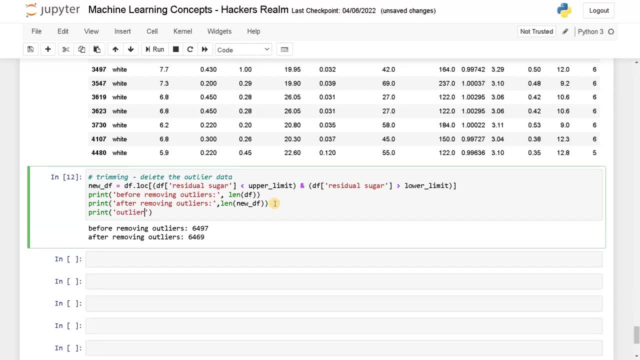 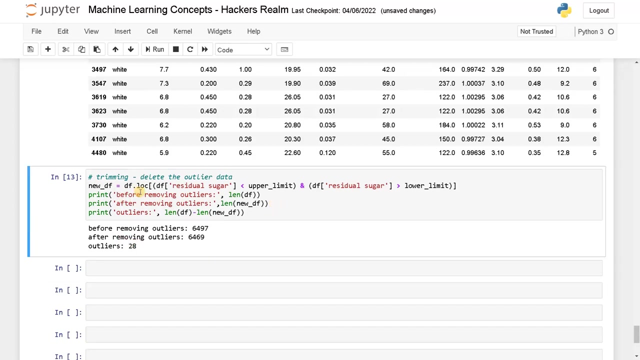 so i'll also have a print statement called outliers equals len of new df and len of old df minus those outliers are Herm, parade r all shall be right. if let's say i'm playing with in this large null Couple of days ago, I just did a product quick analysis and 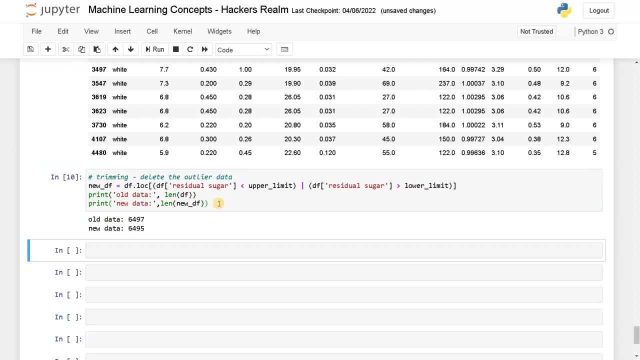 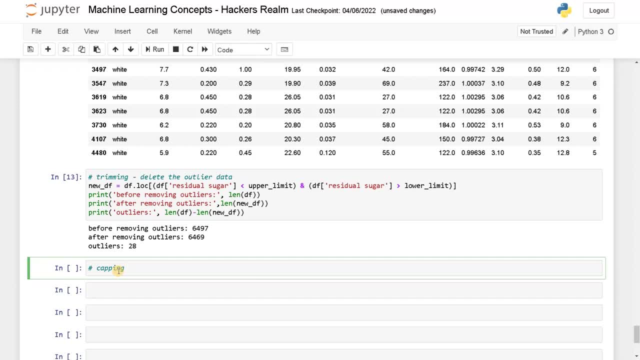 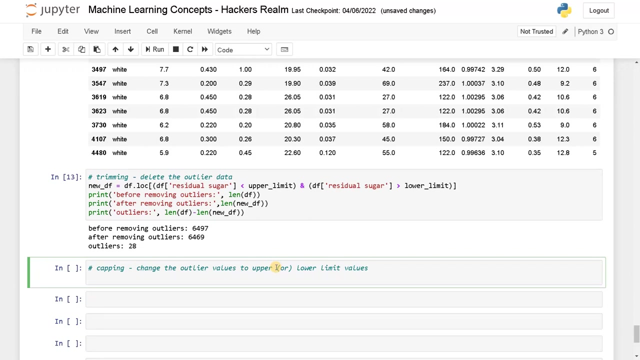 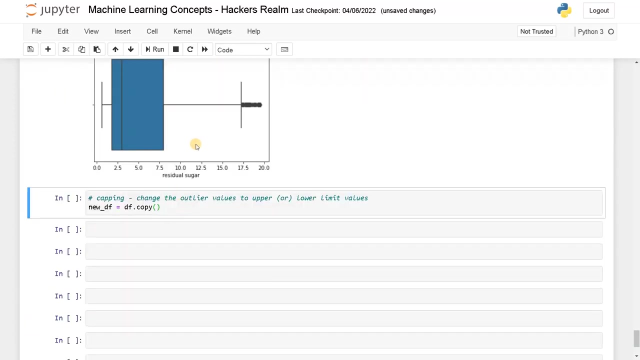 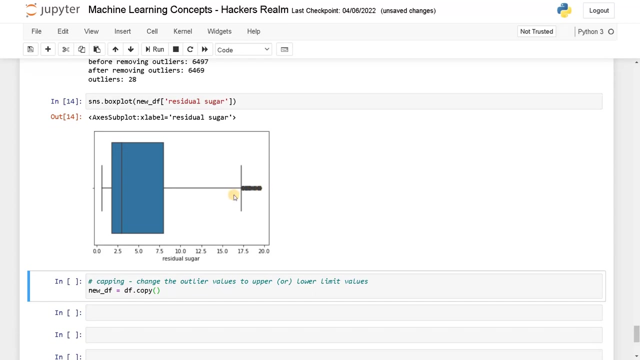 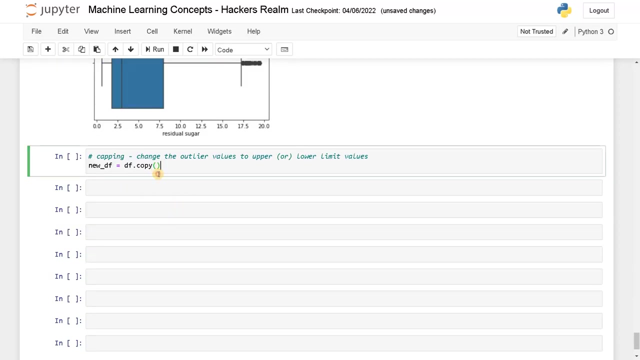 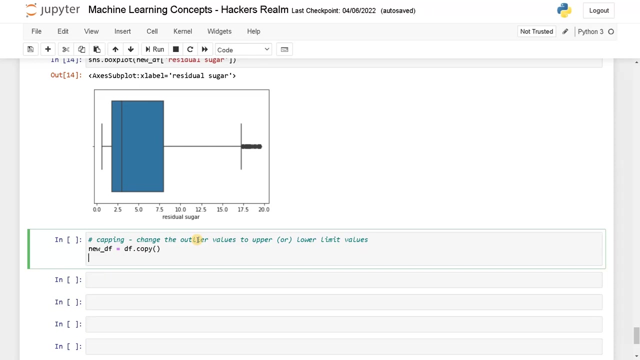 New DF of residual sugar is greater than upper limit and we have to change only the residual sugar column. residual sugar equals upper limit. so what I am doing is I am just filtering out the data which are outliers. that is more than the upper limit value. I am just getting those values and replacing with the upper limit. so this is called capping. we are just capping the data into the limits. so this will do it for the upper limits and we'll do the same for the lower limit, instead of using this. 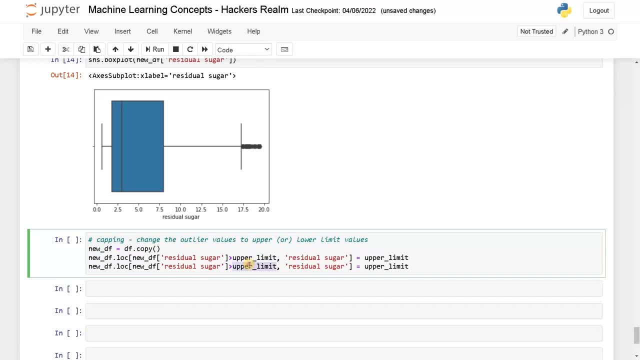 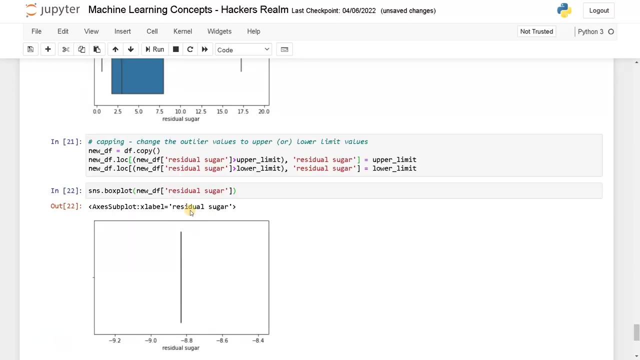 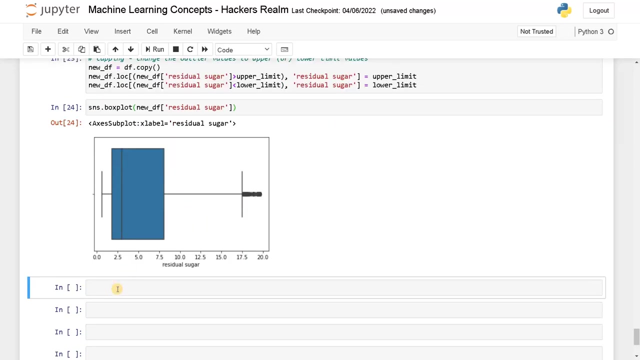 sorry, this will be here. okay, now that's done, let's run this and again, let's display the data. okay, here I have made a mistake. this is less than lower limit. now we can see we have capped the data, so we didn't delete any of the data you. 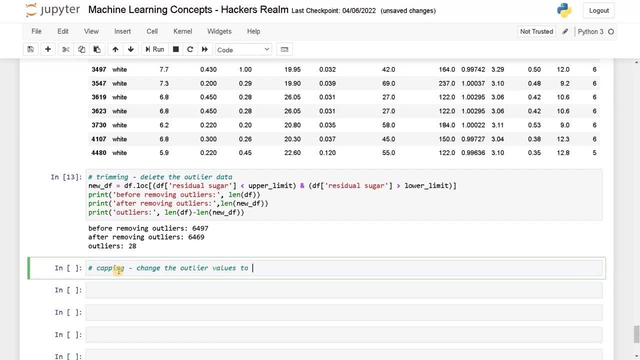 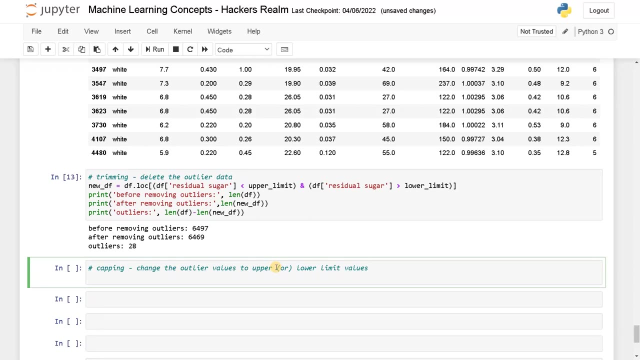 this did not run problem by default and I didn't sometimes know this way of working- or lower limit values. so this is called the capping. if you don't want to delete the whole row, you can do this. so for this i will copy a new data. so df of copy and before doing the capping: 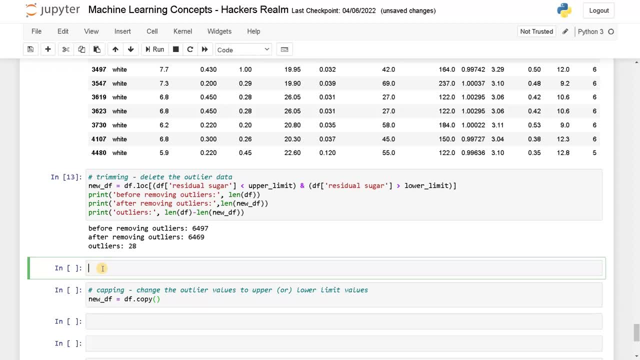 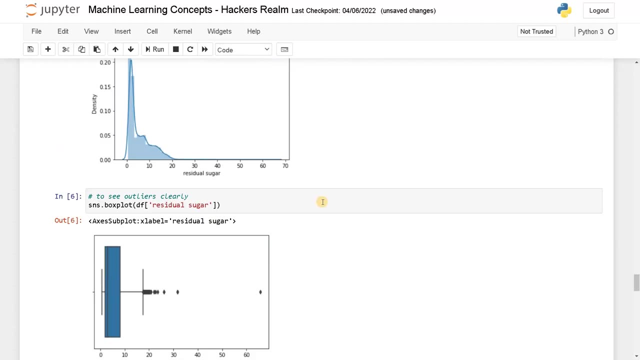 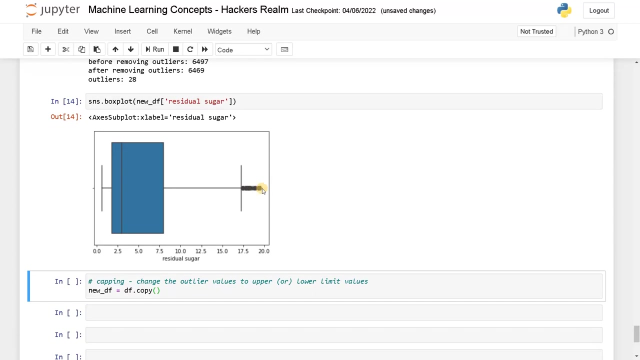 let's also see, uh, how the data looks like after removing the outliers. so sns dot box plot of new df of residual sugar. now you can see the outliers has been removed from this data we are, we have converted to this one, so few other data is there. so this is the allowed outliers, but this is far more better. 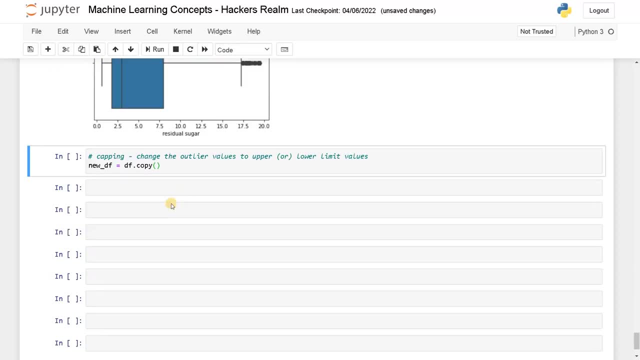 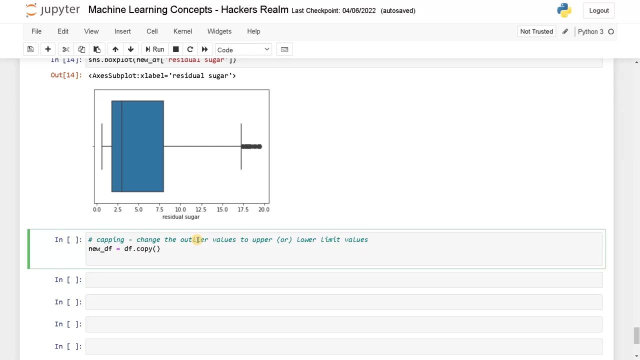 than we have before. so that's good. now let's do the capping part and see how the data looks like. so here, new df dot. location of new df of residual sugar is greater than upper limit and we have to change only the residual sugar in the form of a new df. 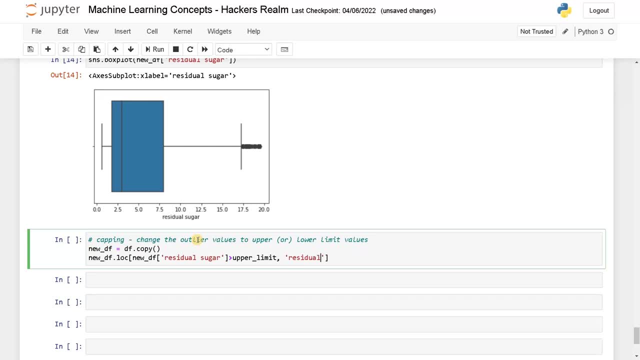 residual sugar column. residual sugar equals upper limit. so what i am doing is i am just filtering out the data which are outliers. that is more than the upper limit value. i am just getting those values and replacing with the upper limit. so this is called capping. we are just capping the data into the limits. so this will do it for the upper limits and 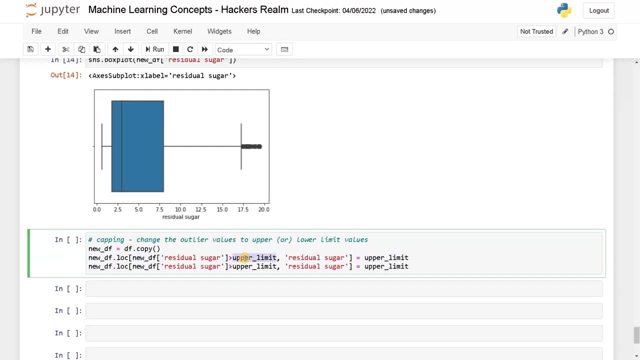 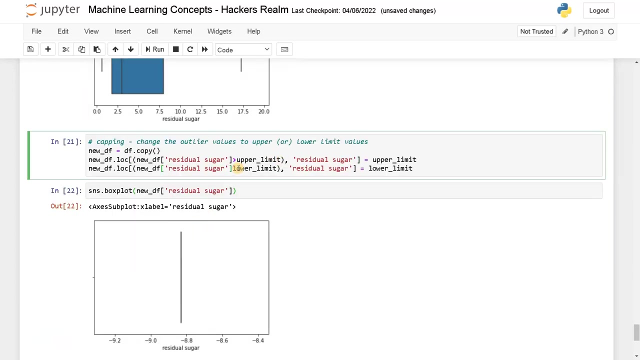 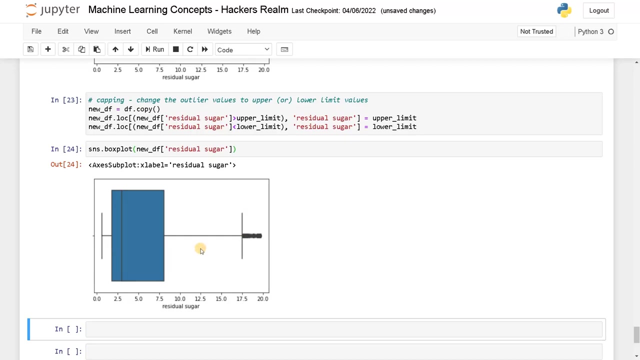 we will do the same for lower limit instead of using this. sorry, this will be here. okay, now that's done, let's run this and again, let's display the data, okay. Okay, here I have made a mistake. this is less than lower limit. Now we can see we have capped the data. 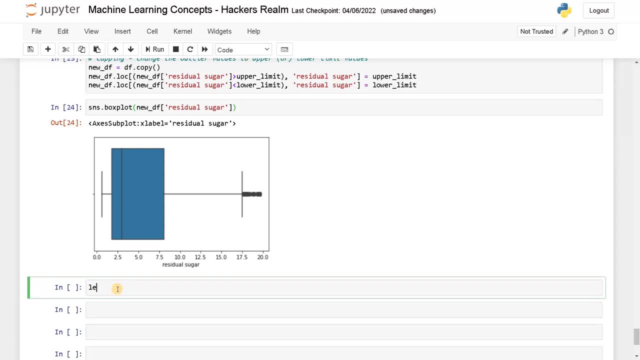 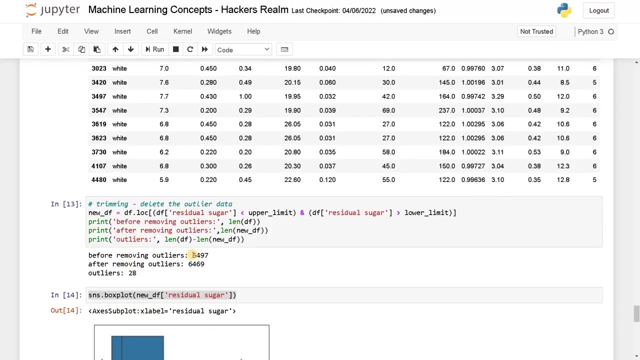 So we didn't delete any of the data. You can check by checking the length len of new df. So this is 6497, that is equal to the old data. We didn't delete it, but we have capped the outliers. 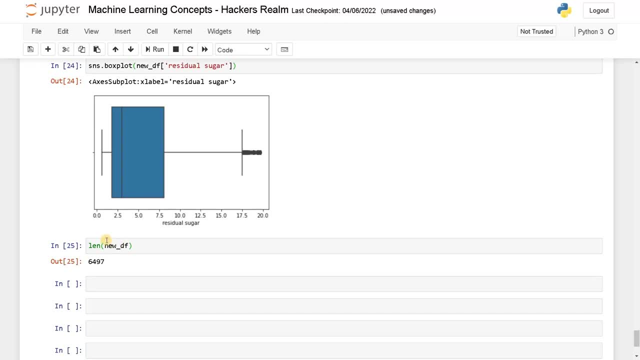 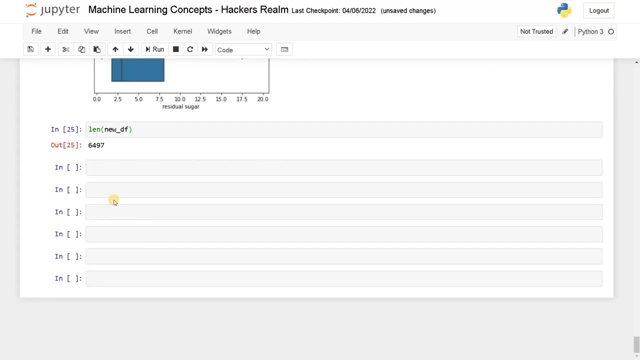 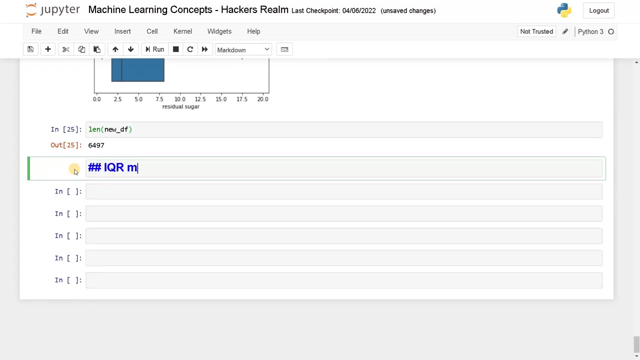 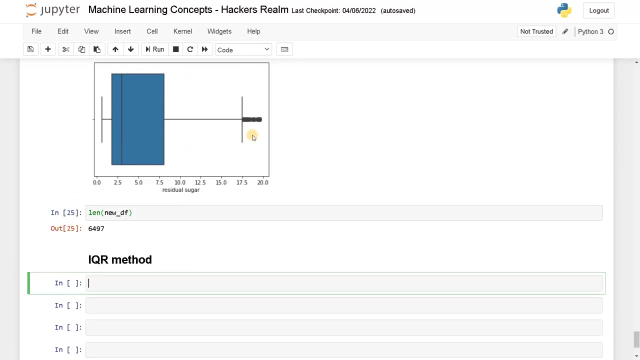 So this is another way of dealing with the outliers. So far we have dealt with zscore method and the next one will be interquartile range method. So interquartile range method. So in the interquartile range method we will be dealing with this boxplot visualization. 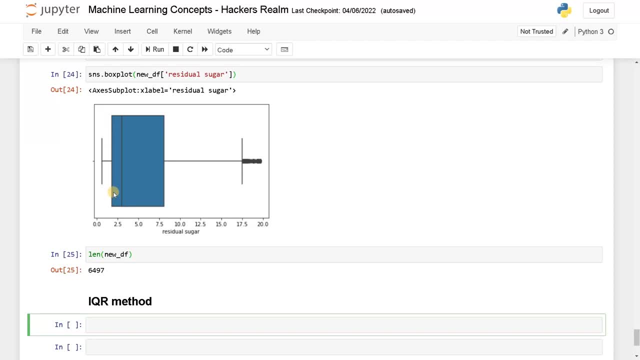 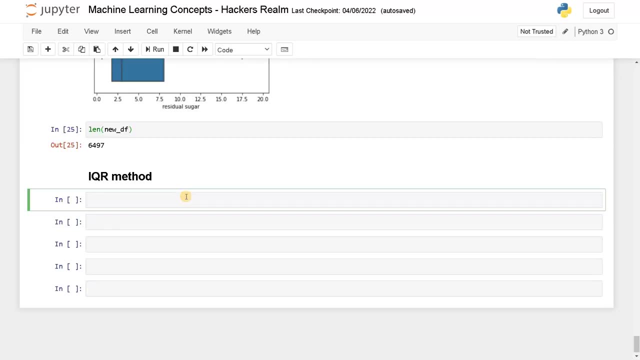 We are going to take the zero point Two, five and zero point seven, five quartile. that is the first and third and multiplies by one point five of the interquartile range. we will be getting a upper limit and the lower limit. 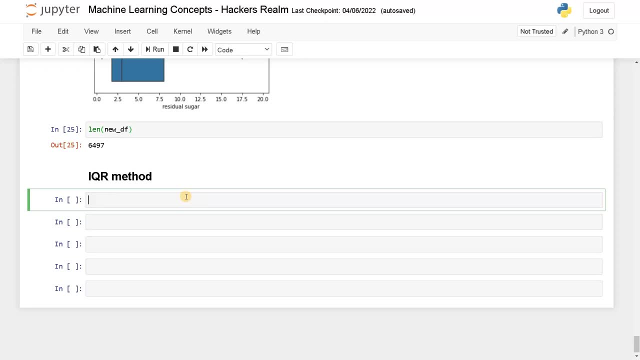 Okay, let's get into it Now. again, I'm going to copy the data. I think we don't need to copy it now. First I will take the q1.. So that will be: q1 equals df- Okay, df of df of residual sugar dot. quantile of zero point two five. 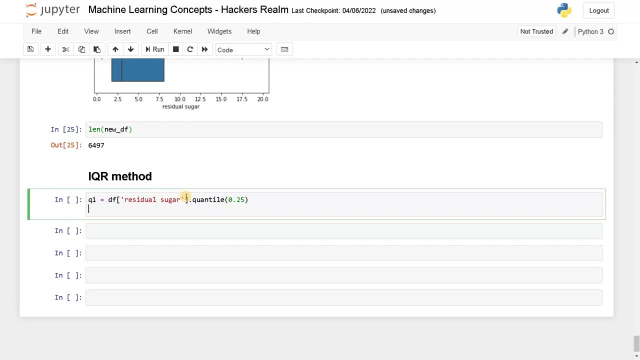 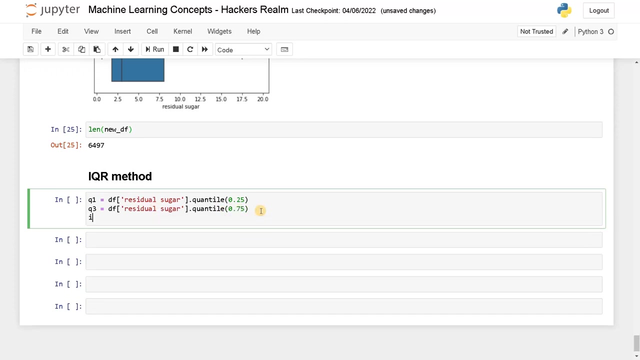 So this is the first quartile and q3. q3 equals again df of residual sugar dot quantile. Here it will be 75.. This is the q3 and to find the interquartile range, iqr equals q1, q3 minus q1. 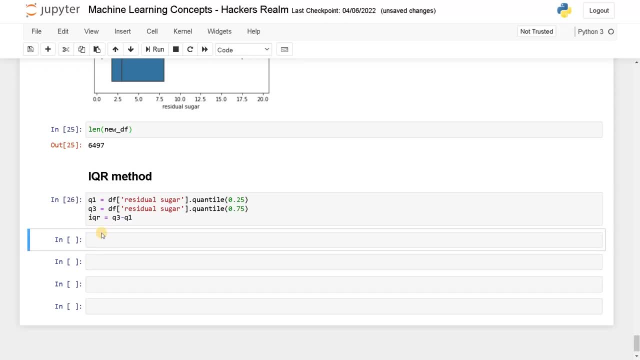 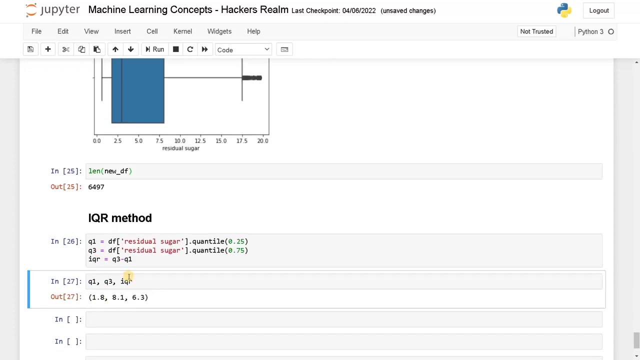 So this is the interquartile range. Let's run this. we'll be getting some values. Let's print that. So print, or just q1, q3 and iqr- Okay, Okay. So this is the first quartile. that is around one point eight, as you can see here, and q3. 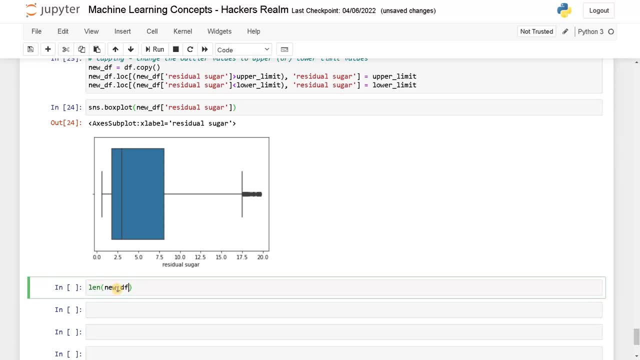 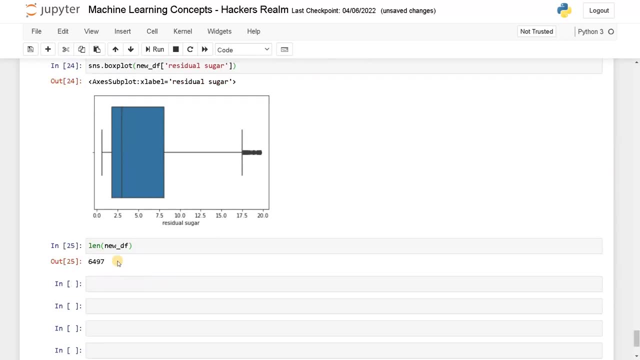 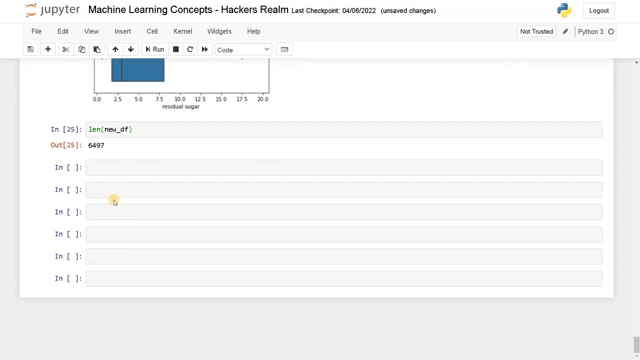 can check by checking the length len of new DF. so this is six, four, nine, seven. that is equal to the old data. we didn't delete it, but we have capped the outliers. so this is another way of dealing with the outliers. so so far we have dealt with Z score method and the next one will be a interquartile range. 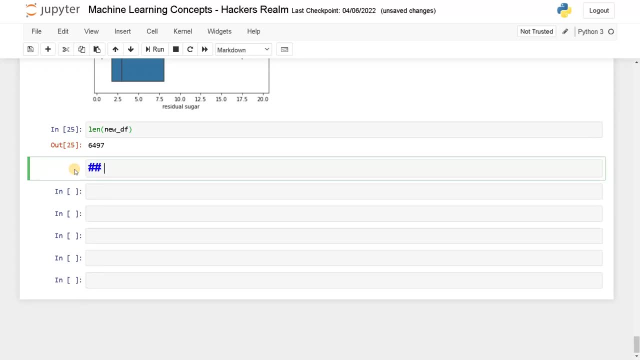 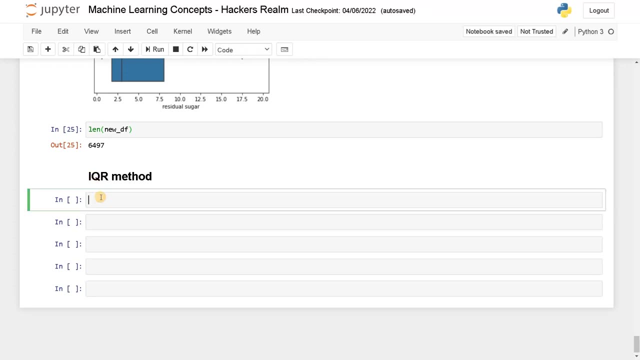 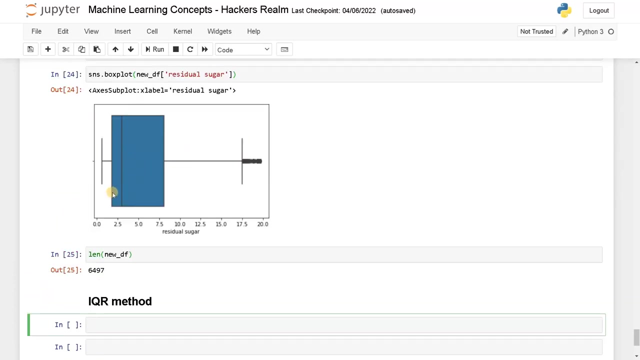 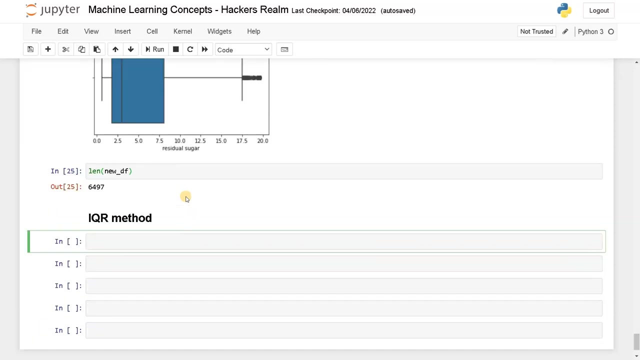 method, so interquartile range method. so in the interquartile range method will be dealing with this box plot visualization. we are going to take the zero point two, five, and zero point seven, five quartile, that is the first and third, and and multiplies by 1.5 of the interquartile range. 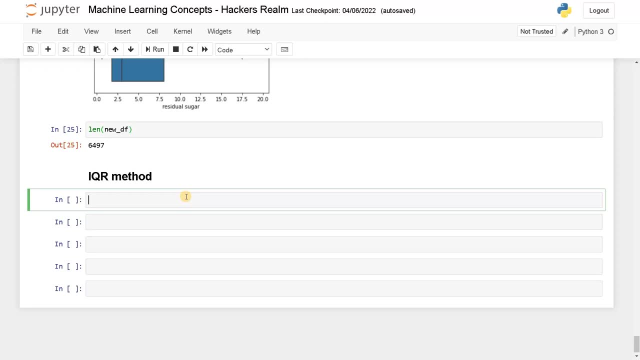 we will be getting a upper limit and a lower limit. Okay, let us get into it Now again. I am going to copy the data. I think we do not need to copy it now. First I will take the Q1.. 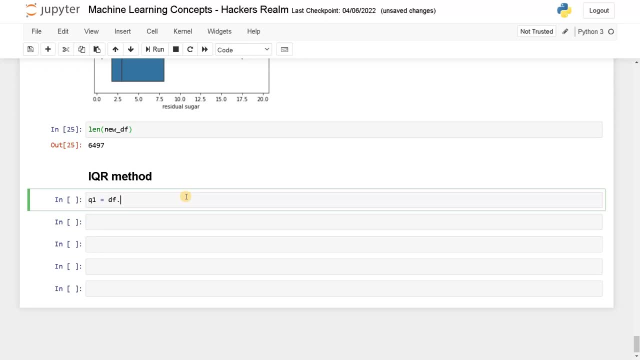 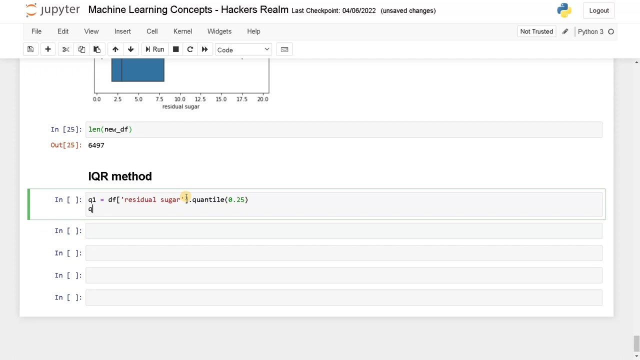 So that will be: Q1 equals DF of residual sugar dot quantile of 0.25.. So this is the first quartile, and Q3 equals, again, DF of residual sugar dot quantile of 0.25.. Here it will be 75.. 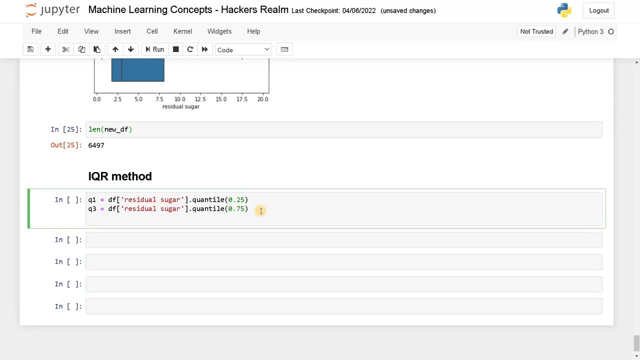 This is the Q3. And to find the interquartile range, IQR equals Q3 minus Q1.. So this is the interquartile range. Let us run this. We will be getting some values. Let us print that. 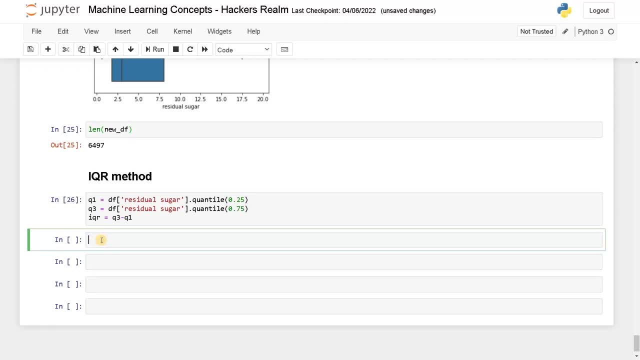 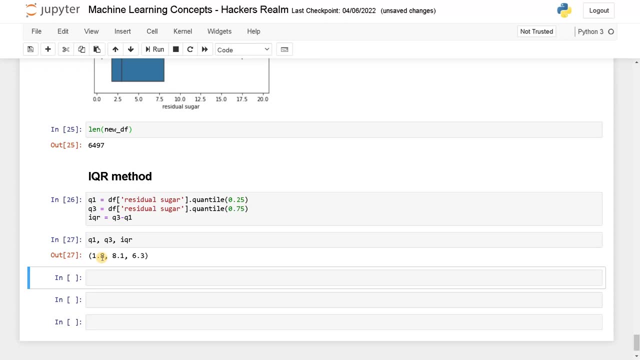 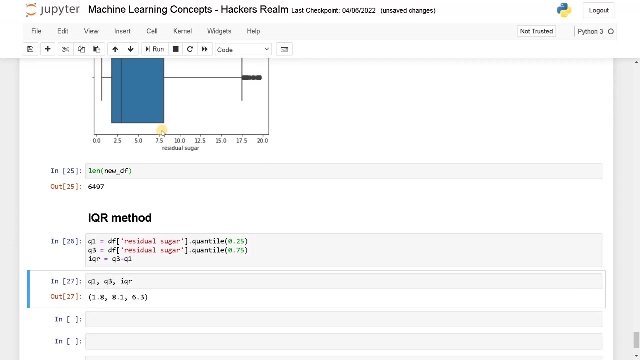 So print just Q1, Q3. And IQR, So this is the first quartile, That is around 1.8,, as you can see here, And Q3, that is 8.1. So that is around here, this edge. 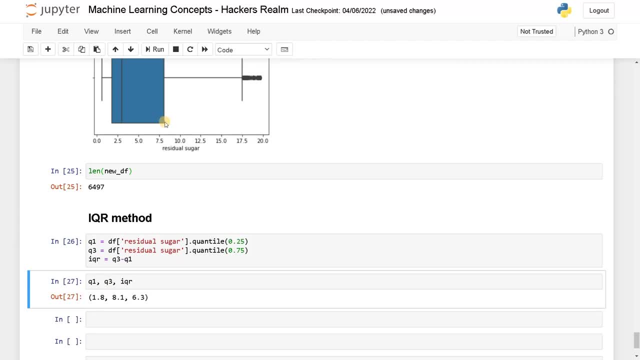 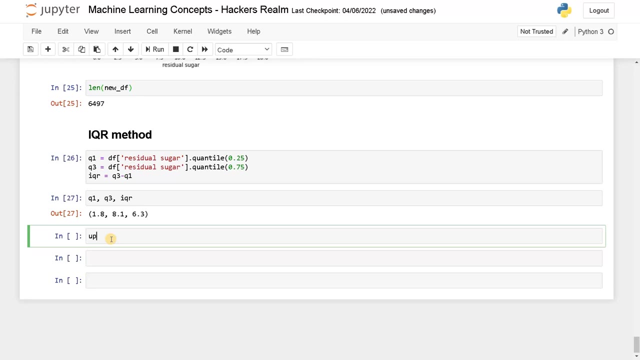 that is eight point one. So that is around here. this edge and the interquartile range is six point three. That is the difference between the quartile one and quartile three. So those are the values. Now we are going to find the upper limit and lower limit again. 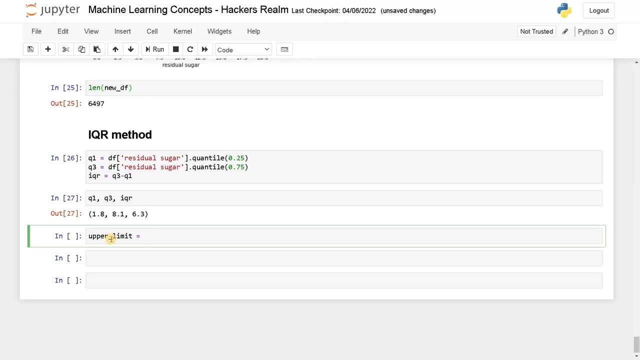 So upper limit equals: Okay, Okay. So that is q3 plus one point five multiplies interquartile range. Now the lower limit, lower limit, equals q1 minus one point five multiplies iqr. So this will give us the possible upper limit and lower limit. 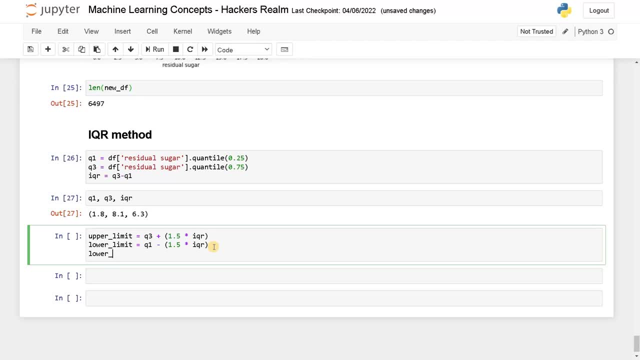 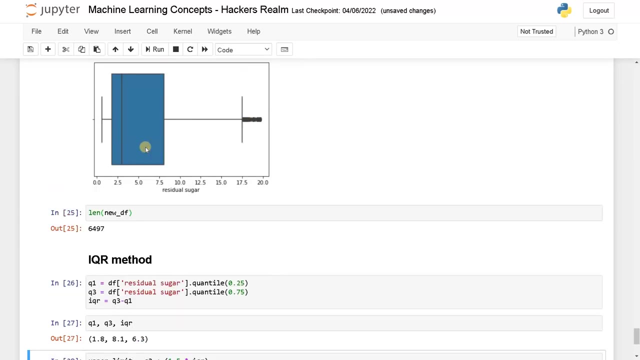 Okay, display those values. so, lower limit per limit. now, as you can able to see, this is the possible lower limit and this is the possible upper limit, as you can see, around 17.5. so this is the line, and here, this is the line, but we have the minimum value around at 0.6. that's why it's not stretching to. 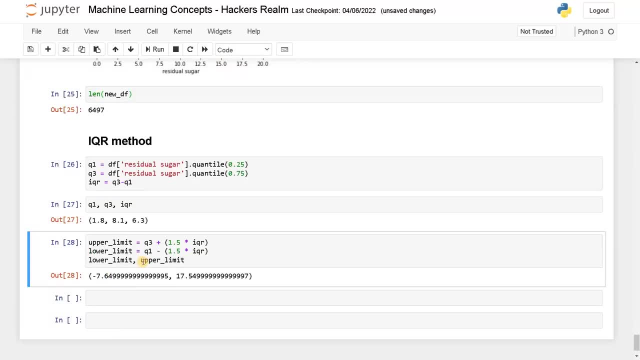 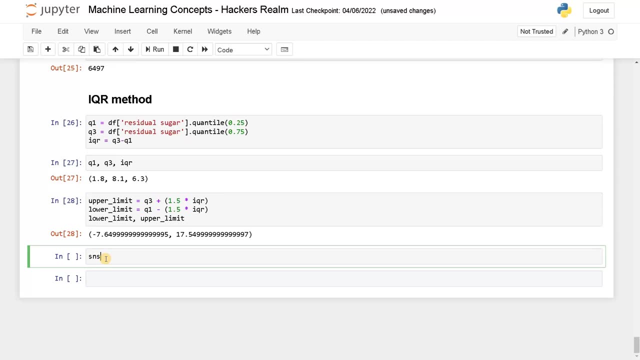 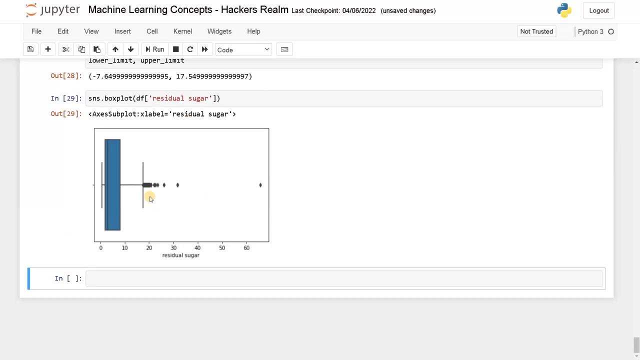 minus 7. the values that is not in the range of this limits can be considered as outliers. so again, i will just plot the data sns dot box plot, because this will be much more better to see the outliers. so here you can see: all these dots will be considered as outliers. okay, let's do the 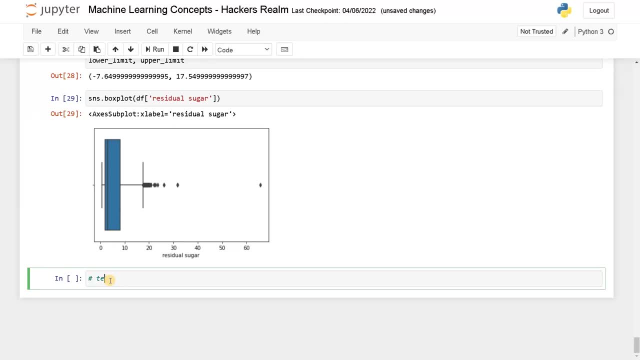 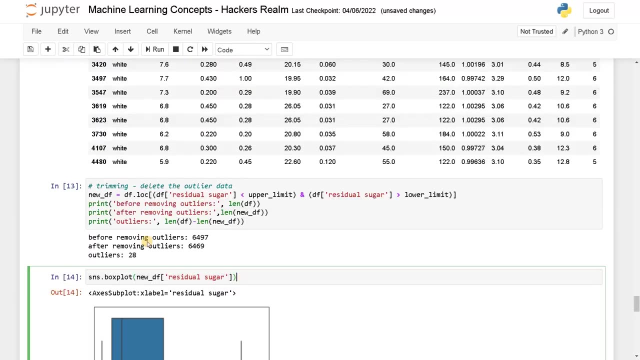 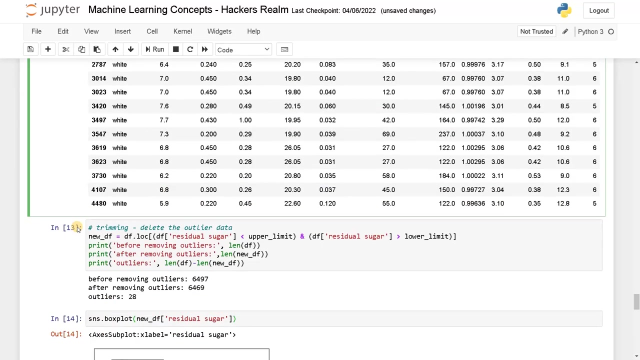 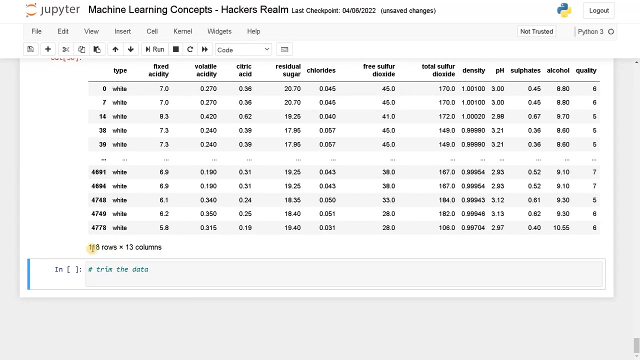 processing again: trim the data. so what we have done before for trimming. so before that, we will just find the outliers. we are using the same values, so we can just copy and paste the code again. so these are the values: around 118 rows has been found. now we will trim the data. 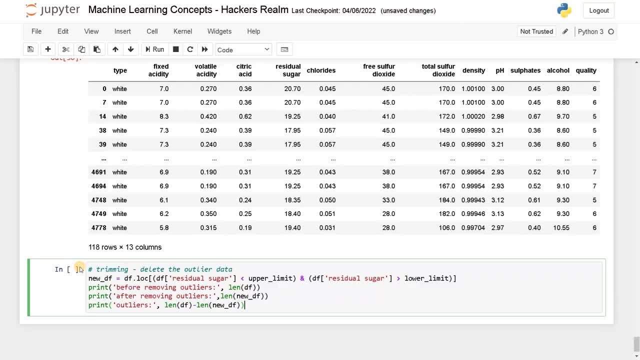 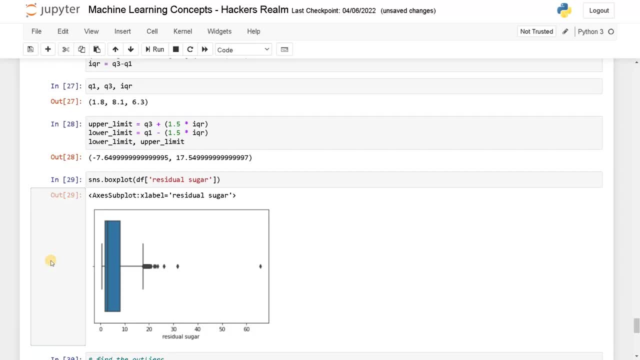 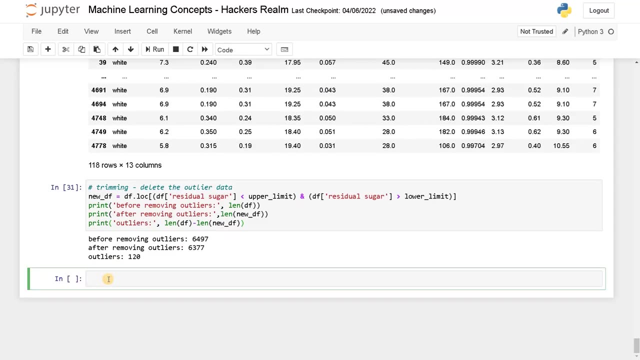 so. so here you can see: 120 outliers has been removed from the data set. now let's do the capping, and also before that i will again show you the plot, how it's changed. so one piece layer to the second layer that is being pulled out. 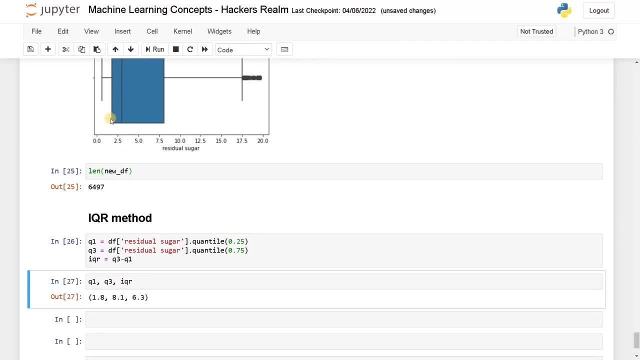 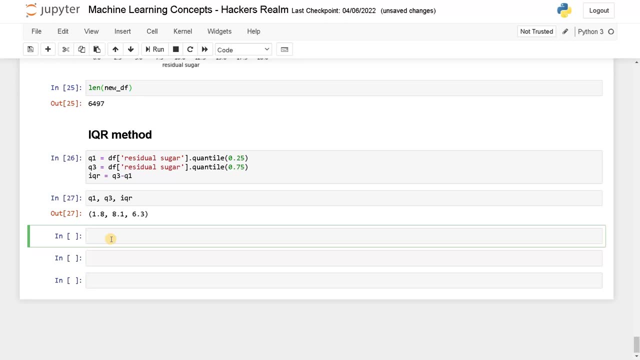 And the interquartile range is 6.3.. That is the difference between the quartile 1 and quartile 3.. So those are the values. Now we are going to find the upper limit and lower limit again. 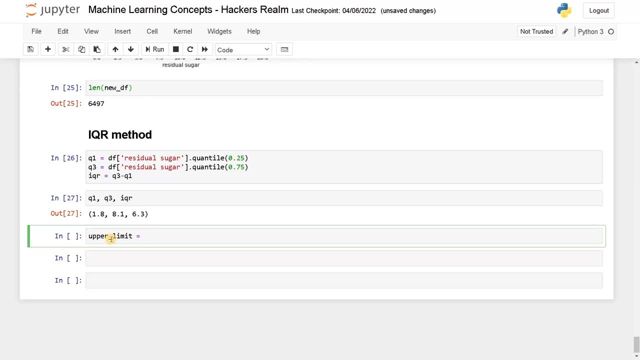 So upper limit Equals Q3 plus 1.5 multiplies interquartile range. Now the lower limit, Lower limit, equals Q1 minus 1.5 multiplies IQR. So this will give us the possible upper limit and lower limit. 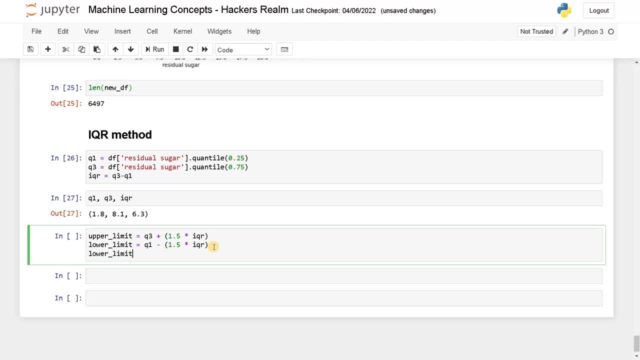 It is also displayed, So let us play those values. So, lower limit, upper limit. Now, as you can able to see, this is the possible lower limit And this is the possible upper limit, As you can see, around 17.5.. 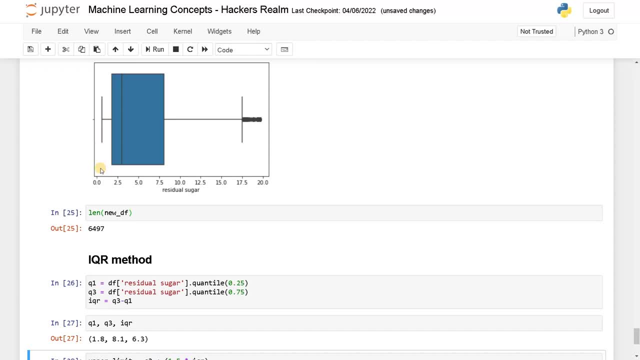 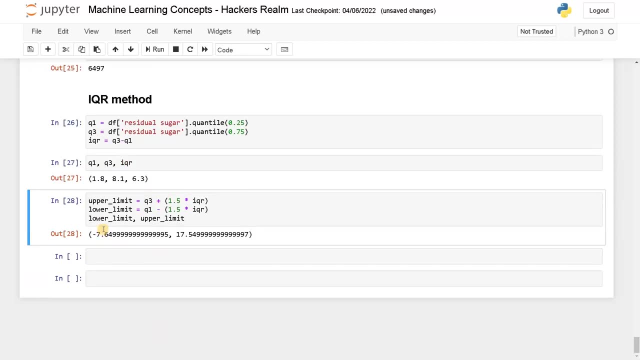 So this is the line, And here this is the line, But we have the minimum value around at 0.6.. That is why it is not stretching to minus 7.. The values that is not in the range of this limits. 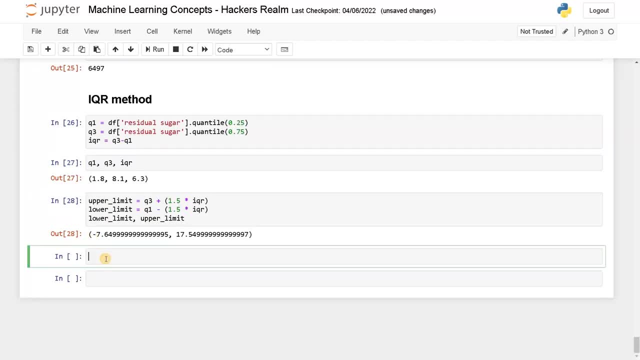 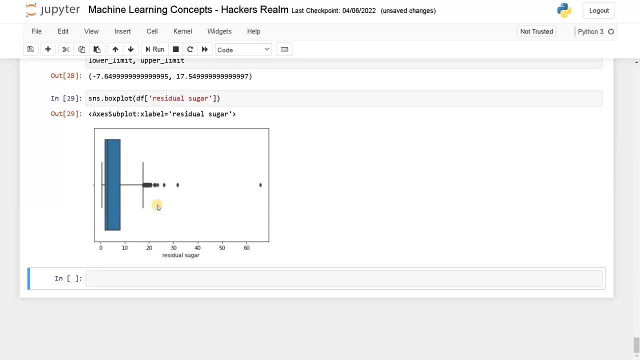 Can be considered as the outliers. So again, I will just plot the data SNS dot boxplot, because this will be much more better to see the outliers. So here you can see: all these dots will be considered as outliers. 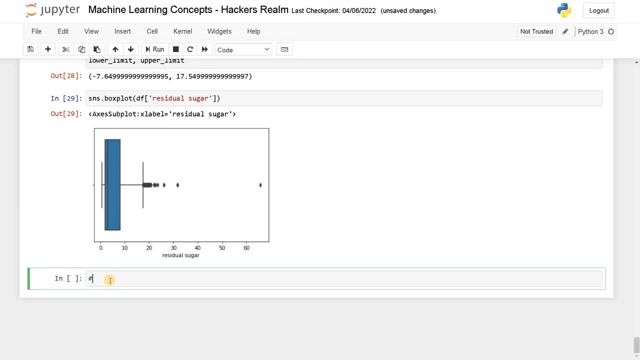 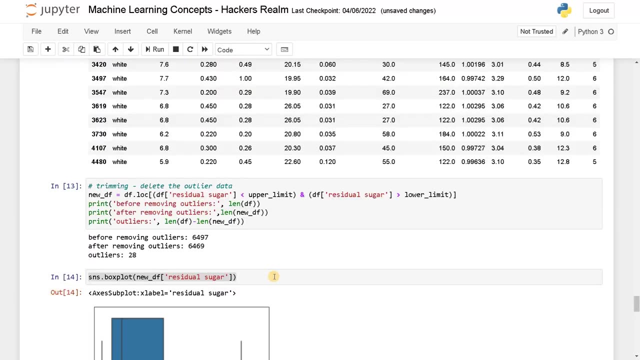 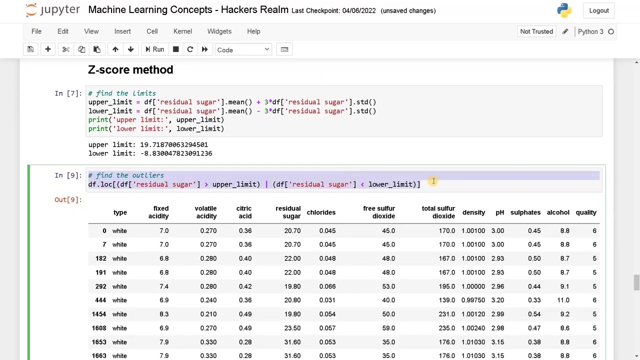 Okay, let us do the processing Again: trim the data. So what we have done before for trimming. So before that we will just find the outliers. We are using the same values, So we can just copy and paste the code again. 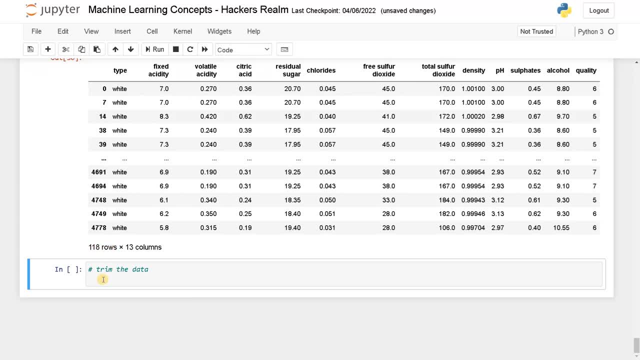 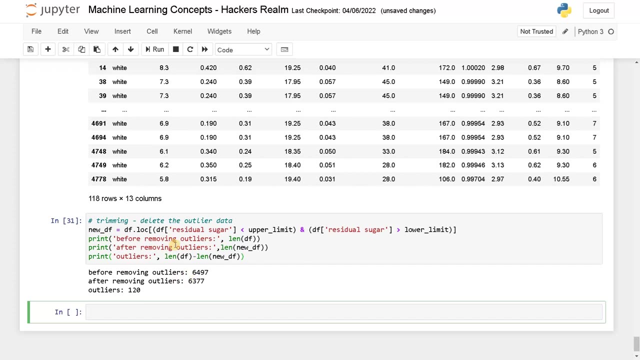 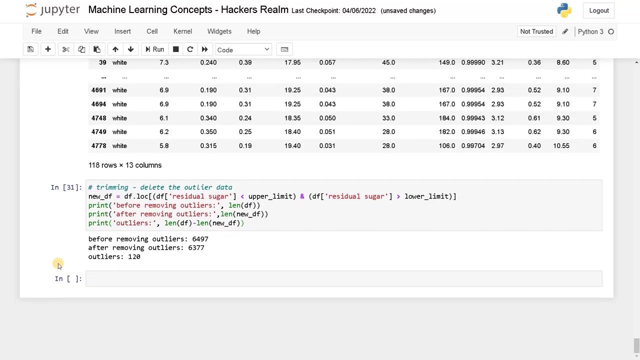 So these are the values. Around 118 rows has been found. Now we will trim the data. So here you can see: 120 outliers has been removed from the data set. Now let us do the capping, And also before that I will again show you the plot. 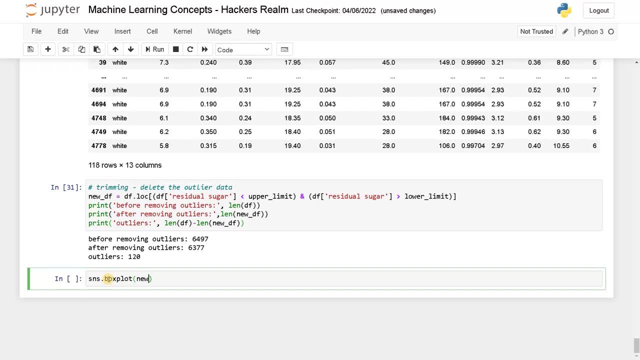 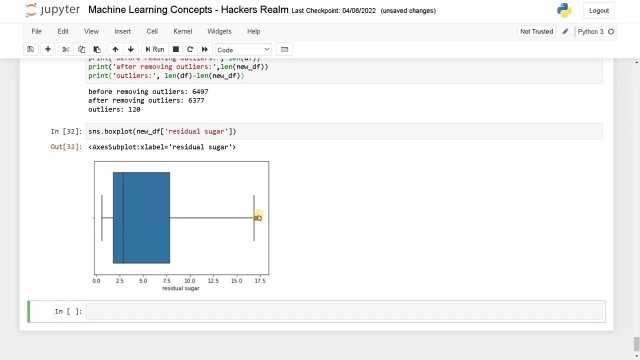 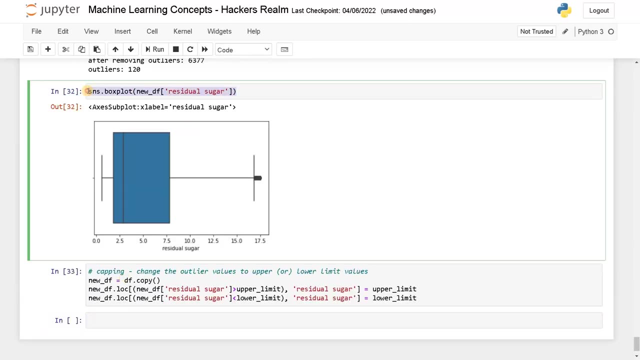 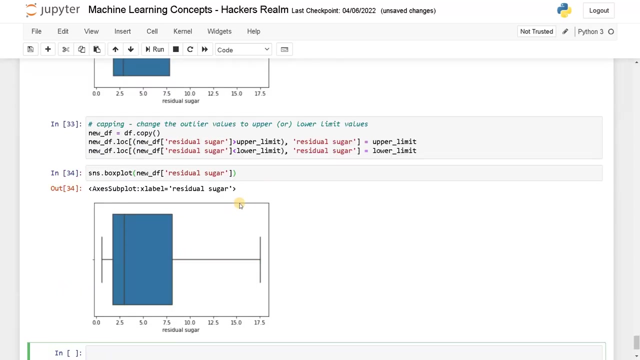 How it is changed. Now you can see all the additional points that are not in the range has been removed Again. we will just do the capping. Plot it again. Now you can see all the values has been capped. 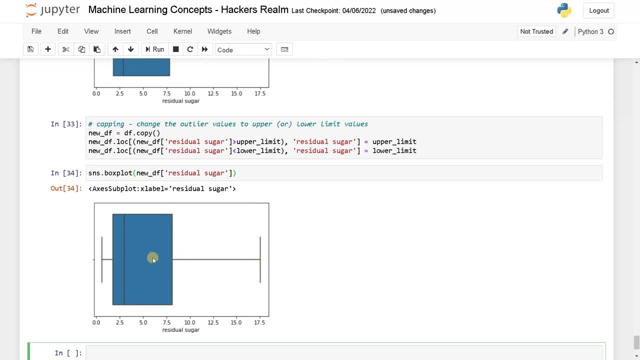 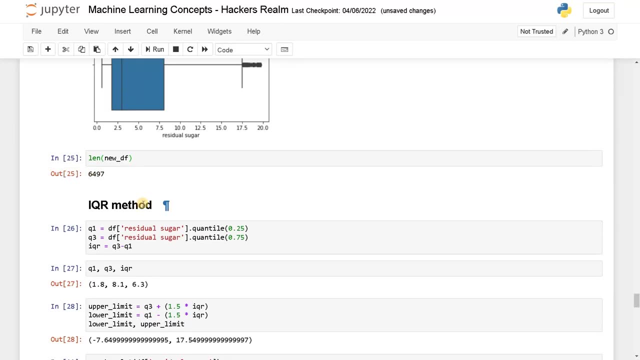 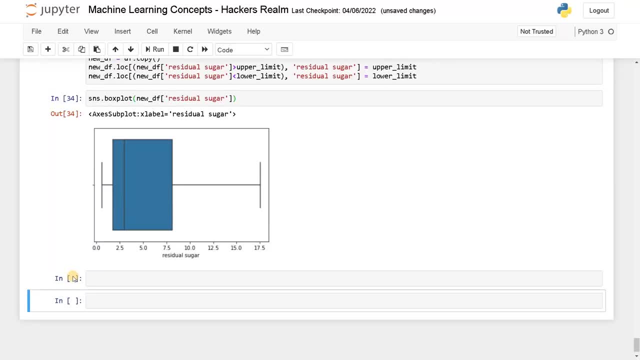 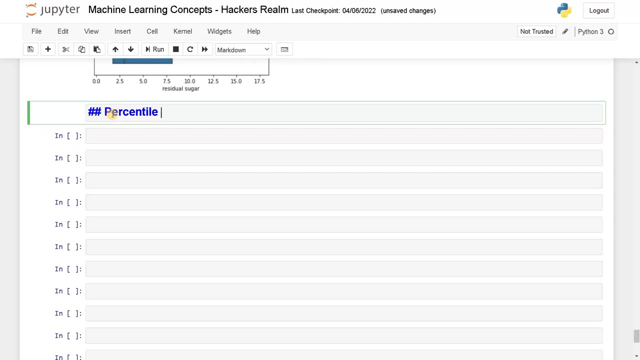 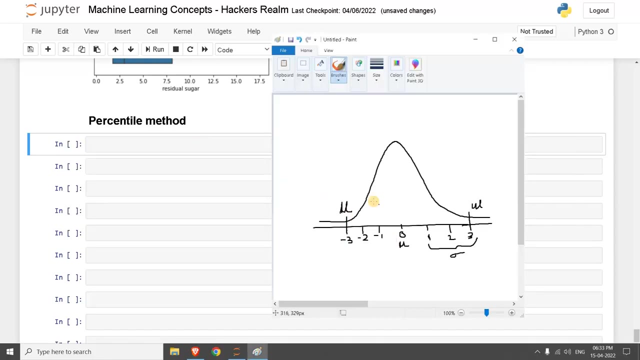 Okay, That is done for interquarting. So that is done for interquarting. Now the next one will be percentile method. So percentile method. So first again, I will explain what it does. So we have drawn a graph like this, right? 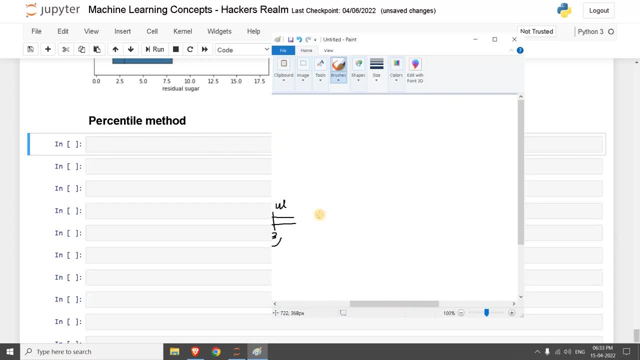 I will just move aside Again. I will just draw a normal distribution. okay, so this is the whole data distribution. what we are going to do is i will just remove the first one percent of the data on the left side. this is around here: 0.1. 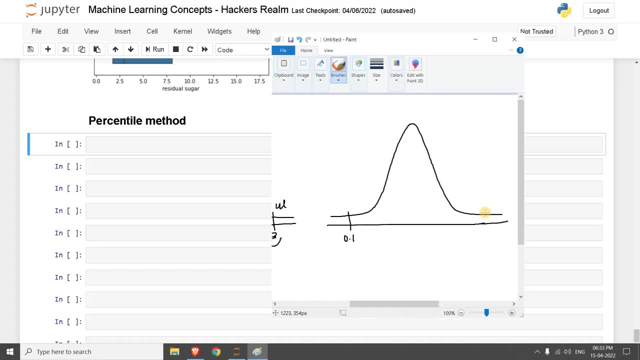 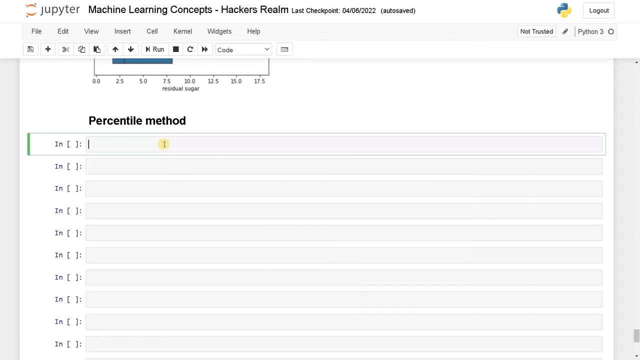 and i'll also remove, uh, the data around like 99 percent, so this will be 0.99. the data that is less than one percent and the data that are more than 99 percent will be considered as outliers and can be removed. so this is called percentile method, again to get the upper. 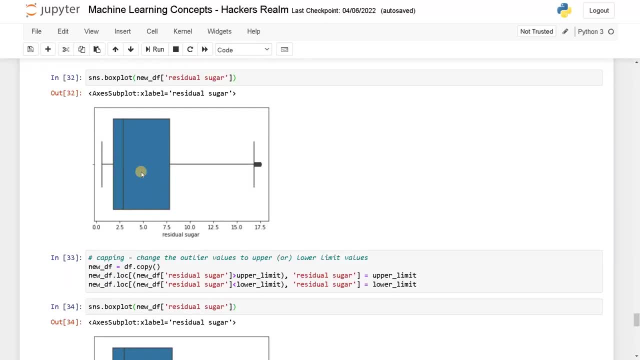 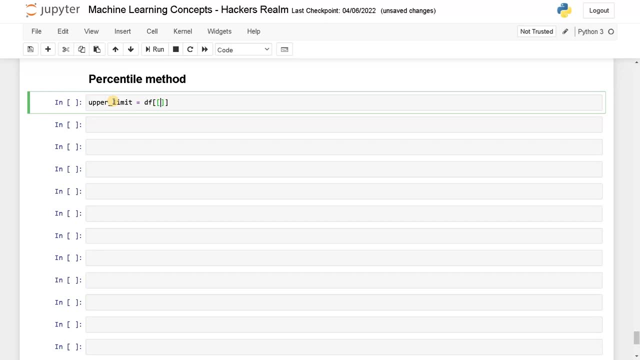 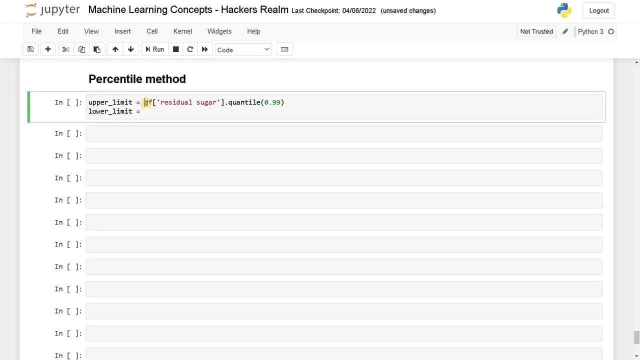 limit and lower limit. we are going to use the quantile, so i can just directly go like this: upper limit equals df of residual sugar, dot quantile. so upper limit will be 0.99. so that is the max possible value. lower limit: again the same syntax, but here it will be 0.01. letters to the symbols of data set, and this is where we will be removing the outliers from the data, as i can here. you can see: 120 layers has been removed from the data set. now let's do the capping also. before that, i will again show you the plot, how it's changed now. now you can see uh game editing. 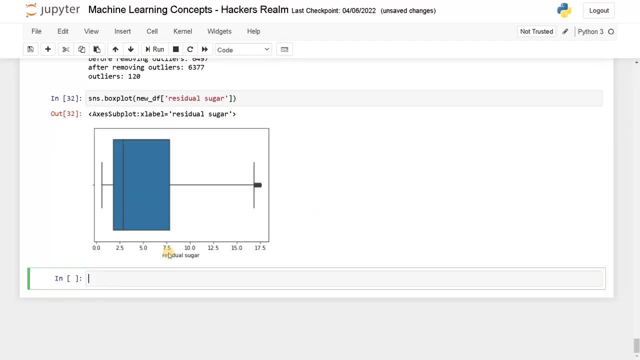 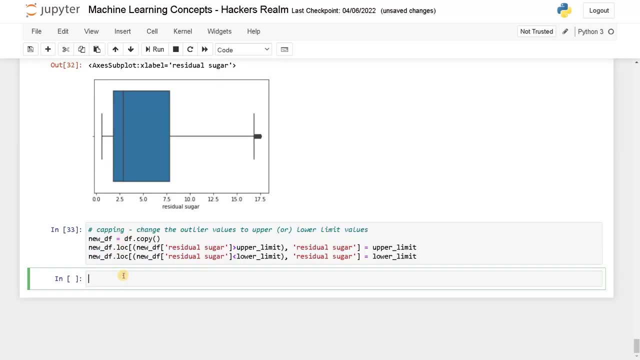 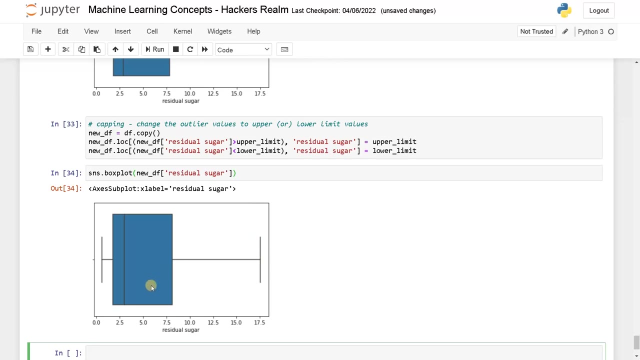 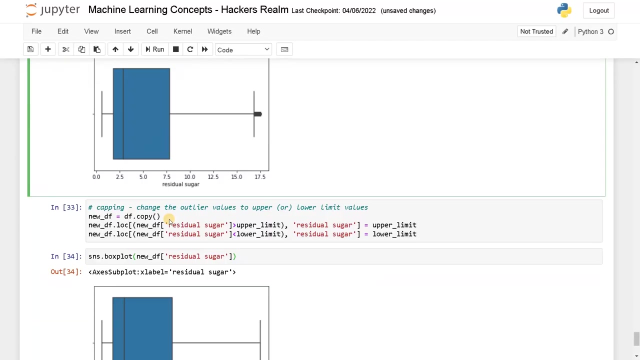 all the additional points that are not in the range has been removed again. we will just do the capping plot it again. now you can see all the values has been capped. so this is a clear box plot without any outliers. so these are the good methods you can apply. okay, that's. 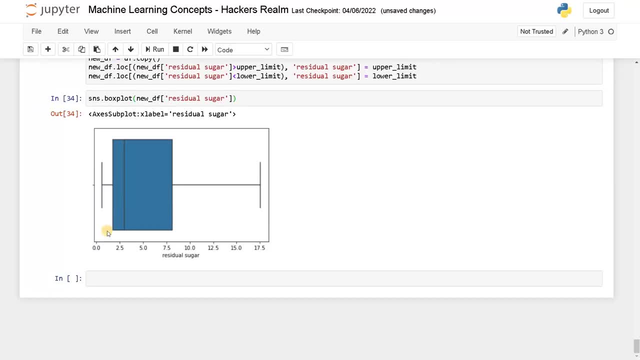 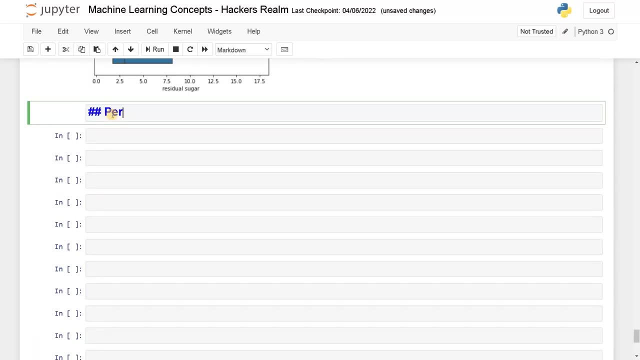 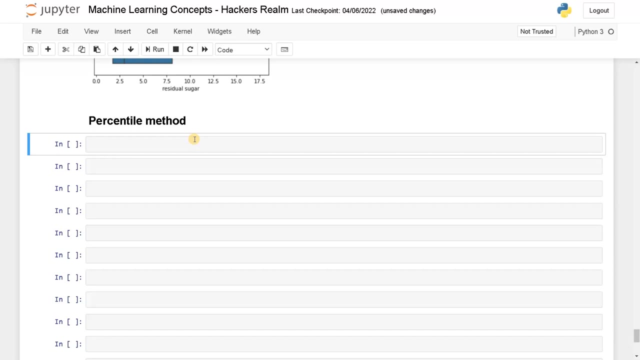 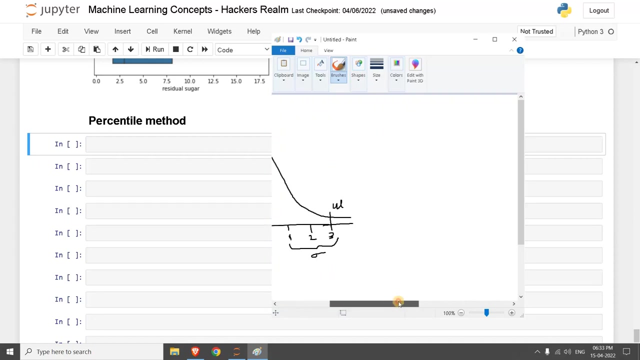 done for interquartile range method. now the next one will be percentile method. so percentile method. so first, again, I will explain what it does. so we have a drawn, a graph like this. right, I'll just aside again, I will just draw a normal distribution you. 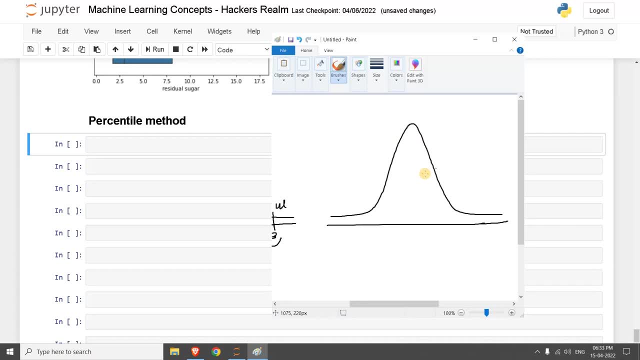 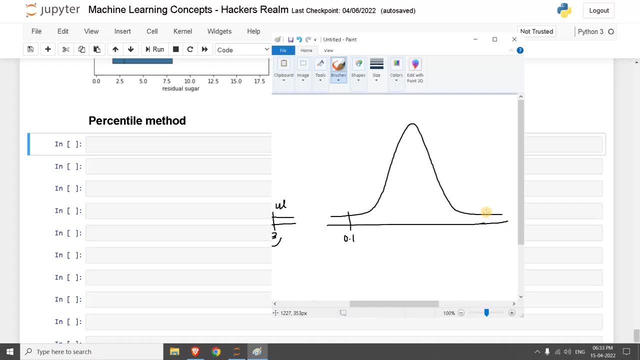 0.1, and I'll also remove the data around like 99%, so this will be 0.99. the data that is less than 1% and the data that are more than 99% is less than 1% of the data. 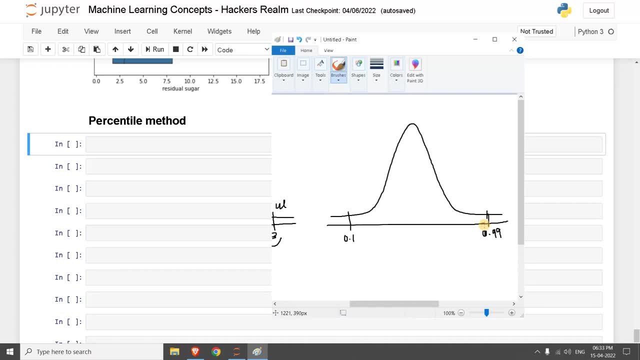 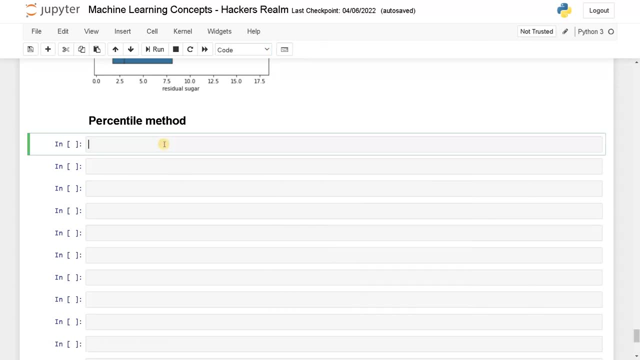 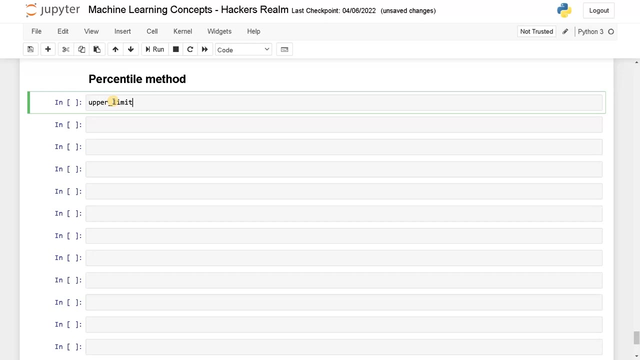 99 will be considered as outliers and can be removed. so this is called percentile method. again, to get the upper limit and lower limit we are going to use the quantile, so i can just directly go like this: upper limit equals df of residual sugar, dot quantile. 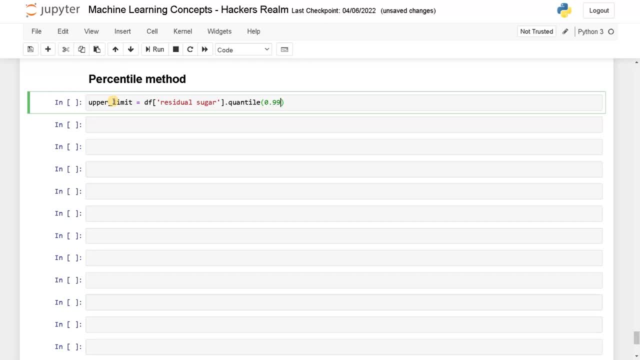 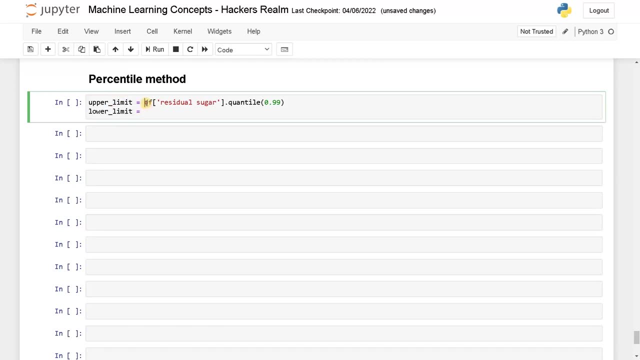 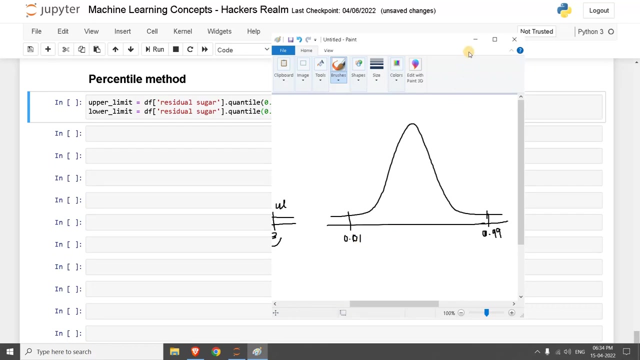 so upper limit will be 0.99. so that is the max possible value. lower limit: again the same syntax, but here it will be 0.01. i think even in the diagram this will be 0.01, denoting the one percent. okay, now we have defined. 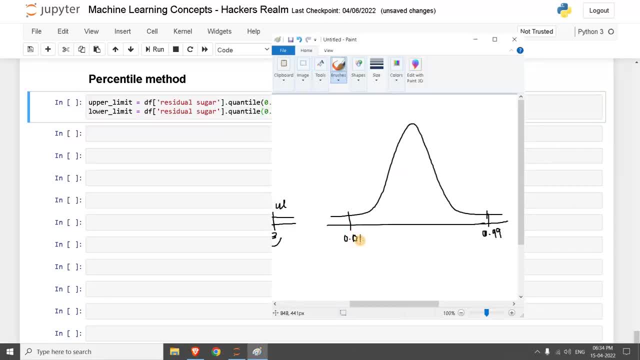 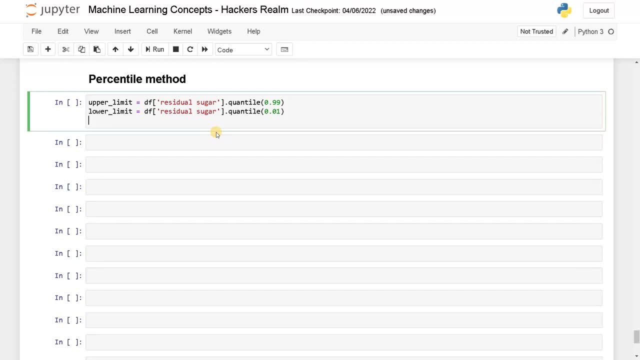 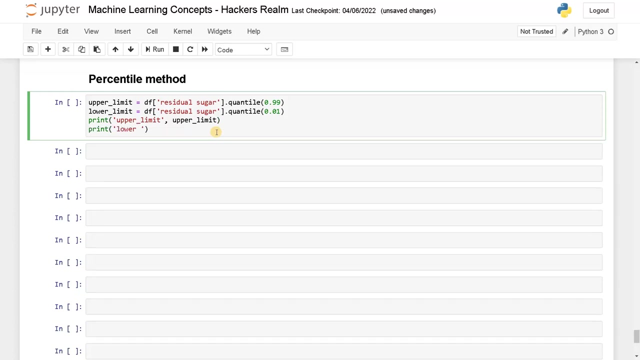 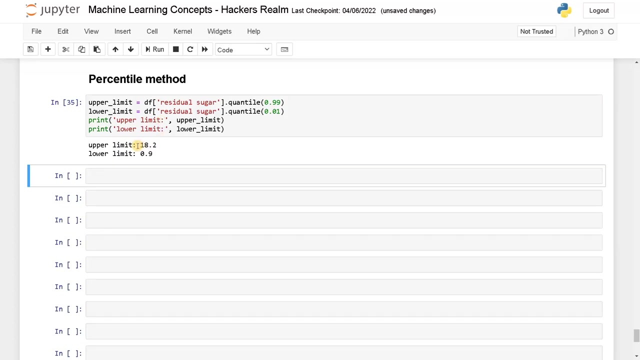 i think even in the diagram this will be 0.01, denoting the one percent. okay, now we have defined the upper limit and lower limit. let's display it. print upper limit again. print lower limit. okay, now you can see. this is the possible upper limit that it allows. 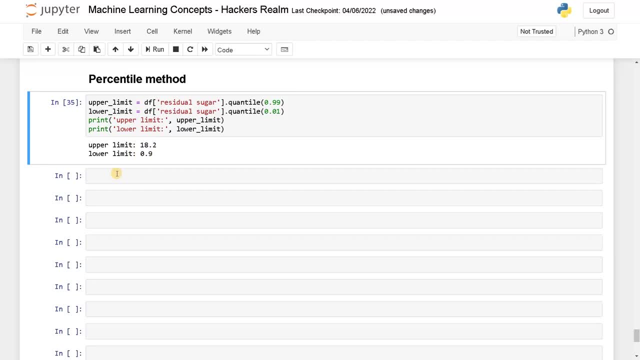 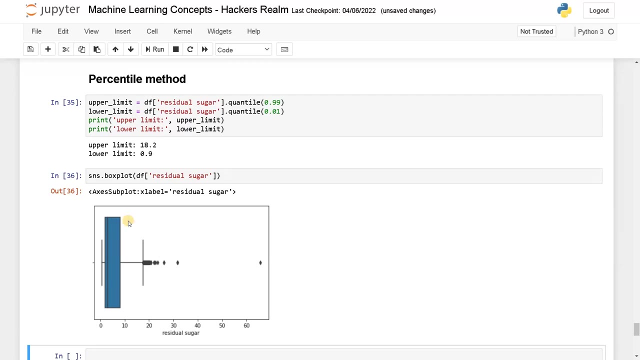 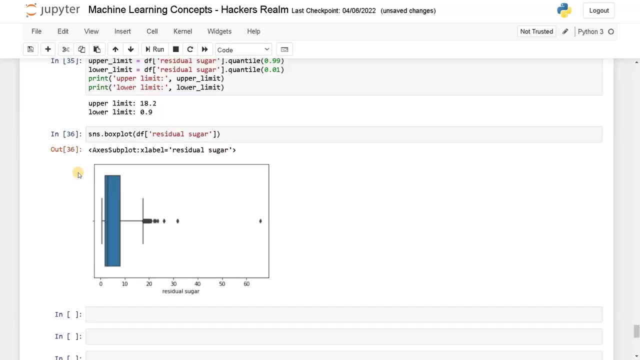 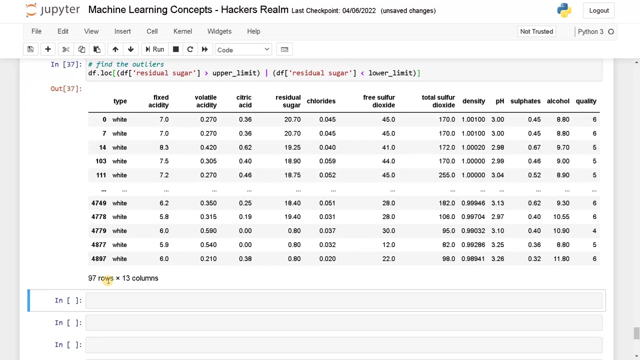 and this is the possible lower limit that it allows. so again, for keeping up with the original data, we will display it. so this is the original data. first, again, let's find the outliers. i'll just reuse the same code. so now it's around like 97, let's trim it. 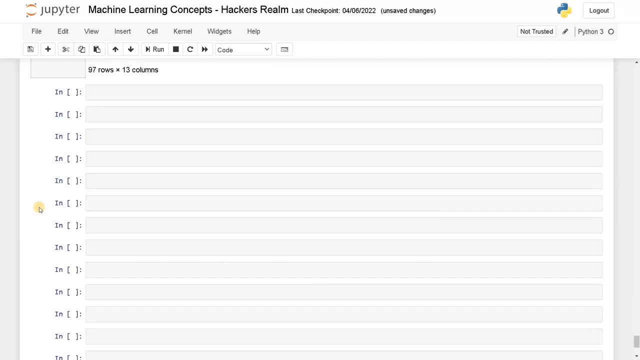 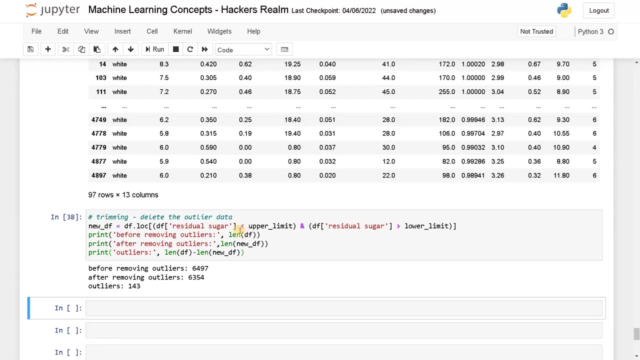 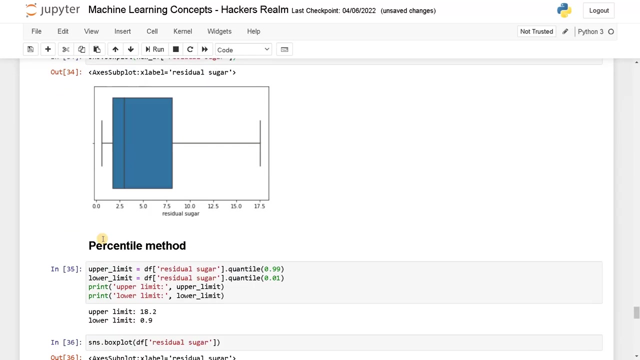 so these are the outliers. that has been removed. you can also set it as greater than or equal to- sorry, less than or equal to in order to uh do this. so this will allow the upper limit as well. maybe i can do the same thing in the above representation as well. 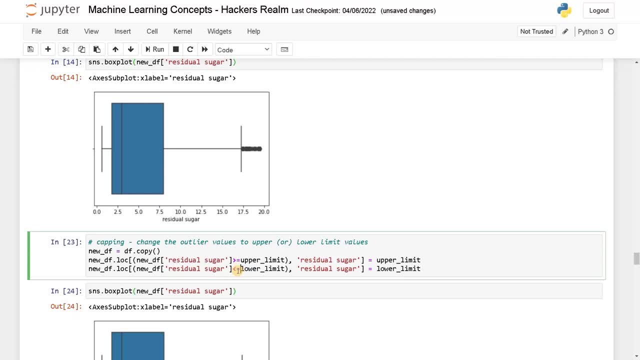 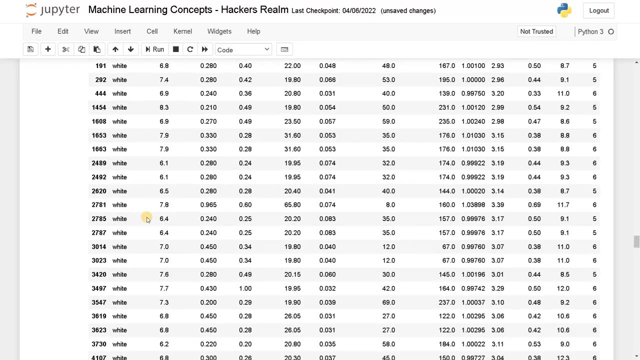 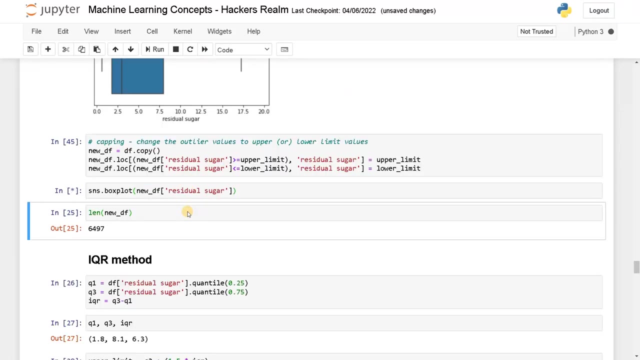 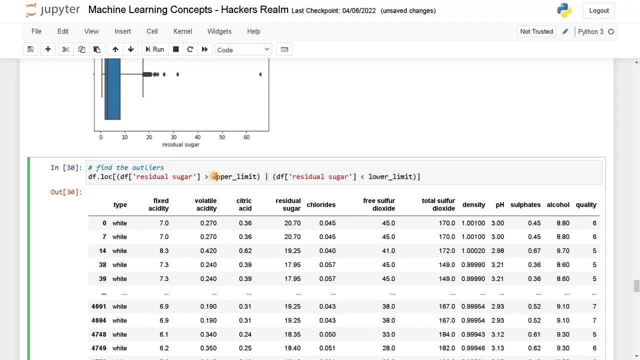 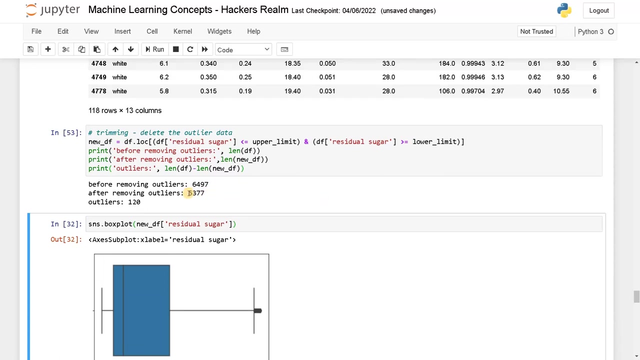 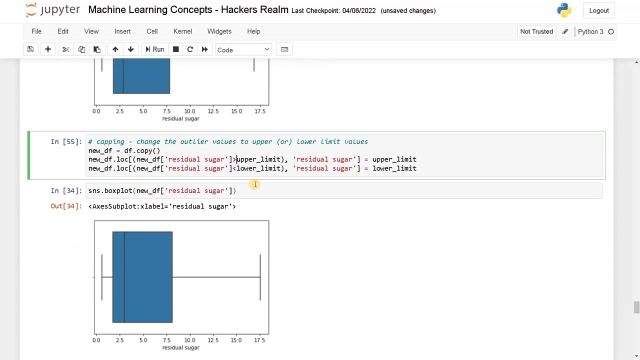 and here also i can do the same, so i'll just run this once again. it's not showing the number of layers now. here it is around 28. okay, this is done, and here also we will do the same. around 120 has been removed, so just adding it more till the perfect level. 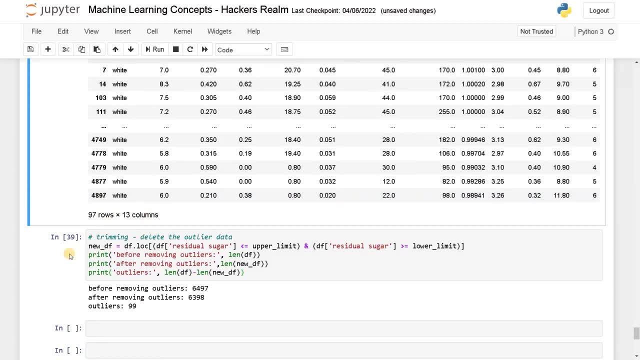 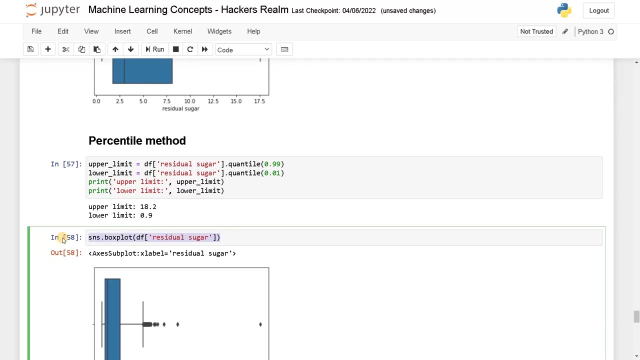 now for the percentile. here you can see around 97. so it removed around like 99 outliers. so it removed around like 99 outliers and this is the data we are getting after removing the outliers. now let's do the exploration again. now let's do exploring again. 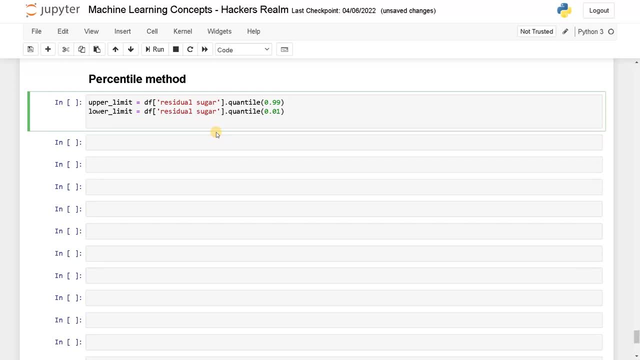 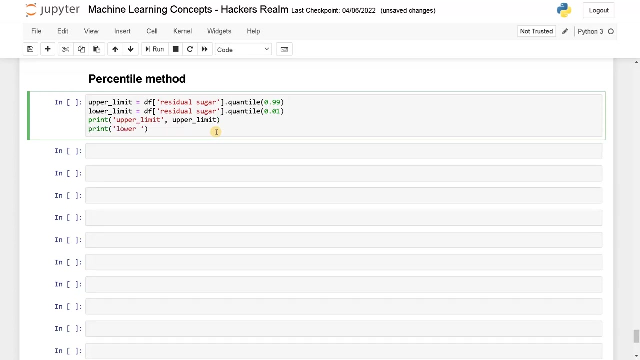 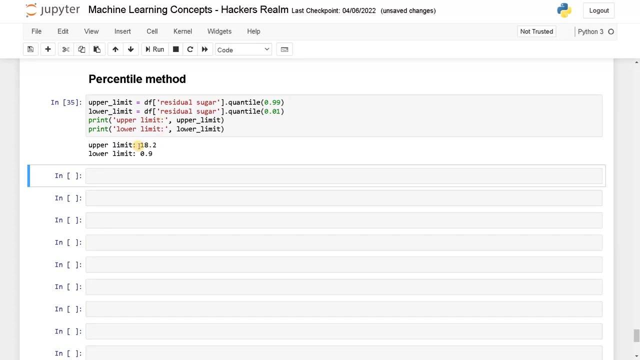 the upper limit and lower limit. let's display it. print upper limit again. print lower limit. okay, now you can see this is the possible upper limit that it allows and this is the possible lower limit that it allows. so, again, for keeping up with the original data, we will display it. 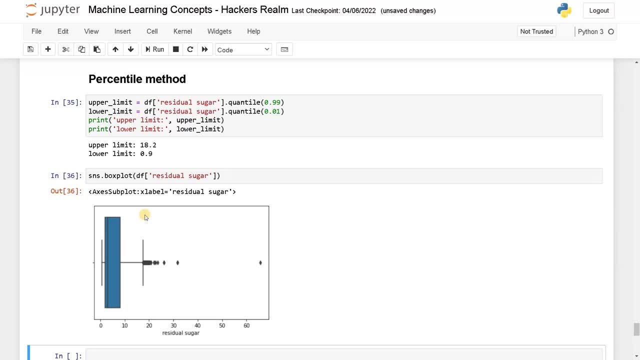 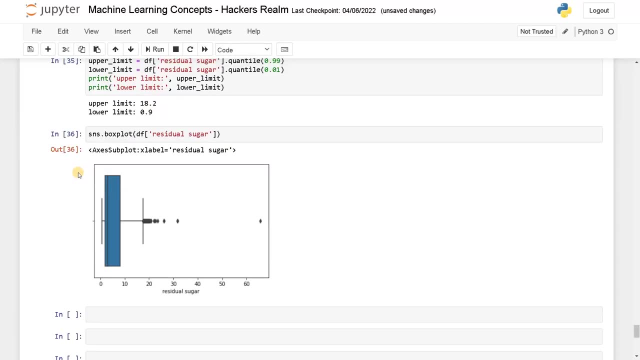 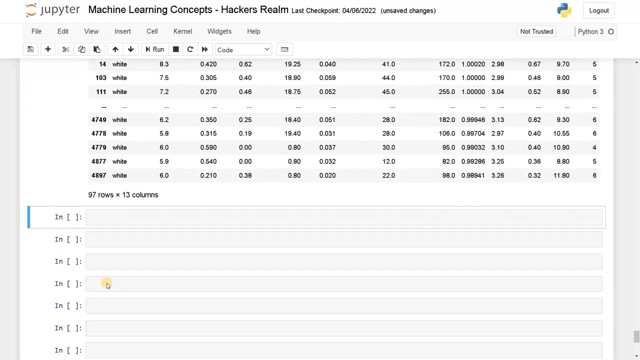 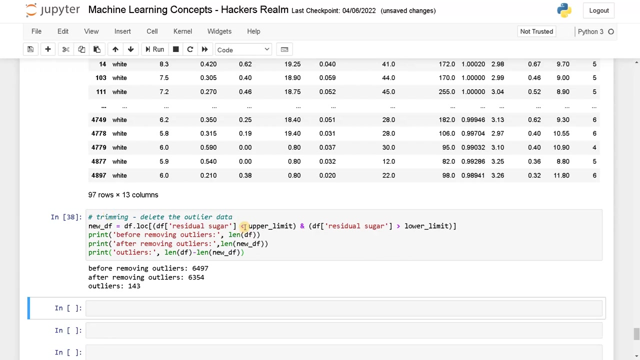 so this is the original data. first, again, let's find the outliers. i'll just reuse the same code. so now it's around like 97, let's trim it. so these are the outliers. that has been removed. you can also set it as greater than or equal to- sorry, less than or equal to, in order to 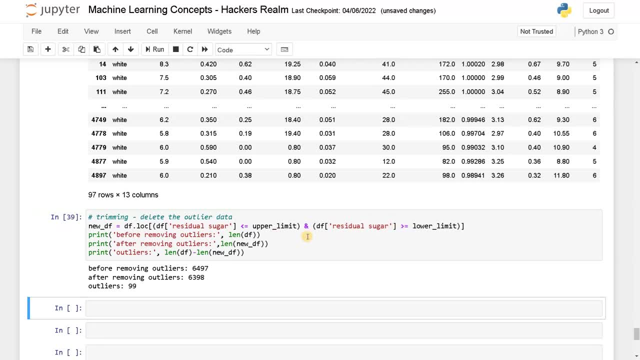 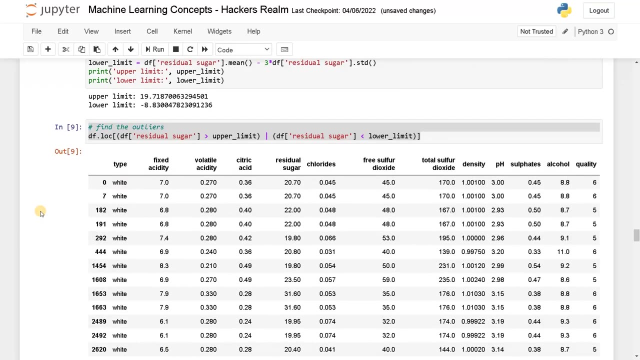 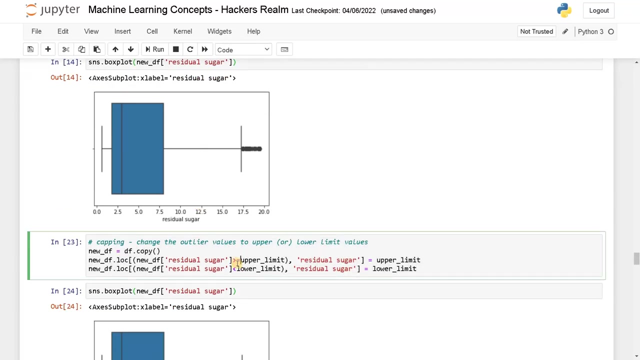 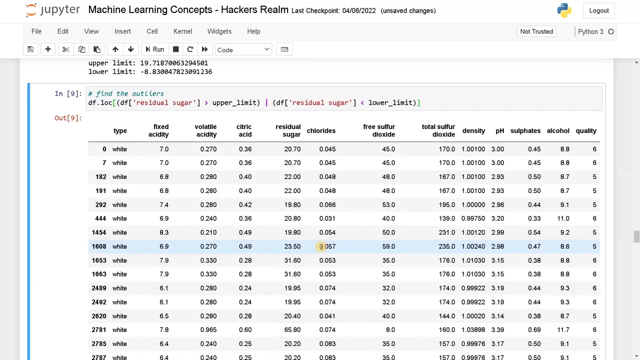 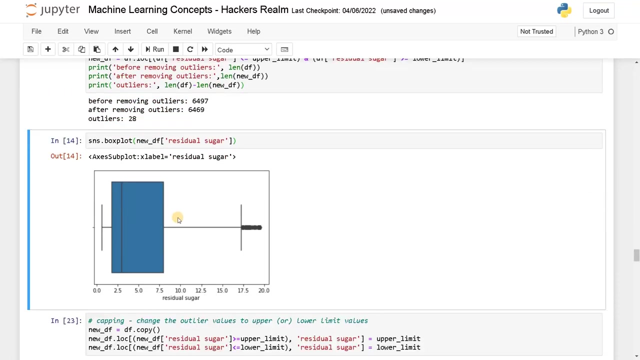 do this, so this will allow the upper limit as well. maybe I can do the same thing in the above representation as well, and here also I can do the same, so I will just run this once again. it is not showing the number of layers. now here it is around 28.. 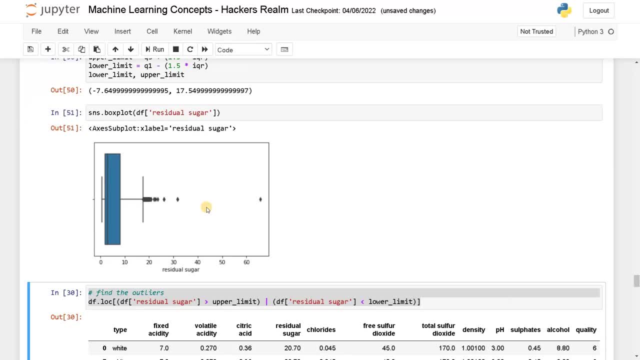 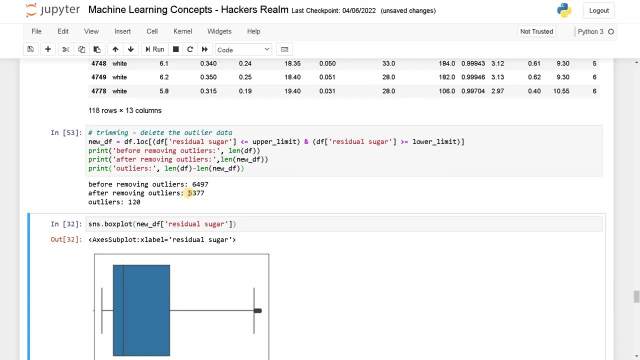 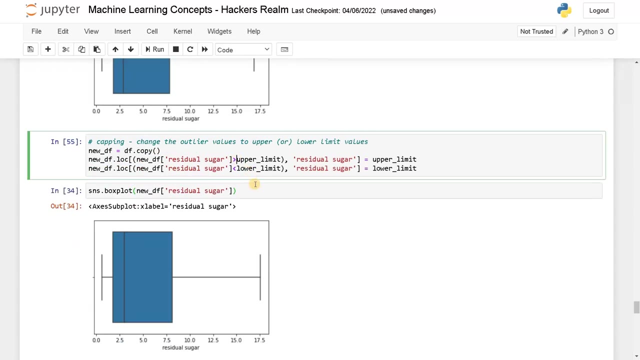 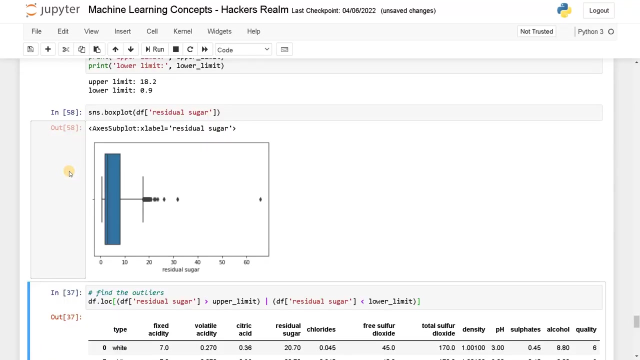 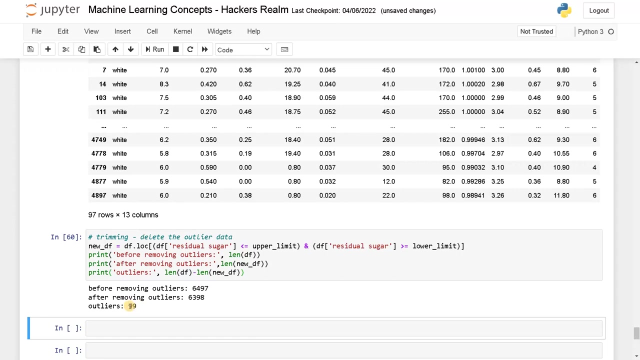 This is done And here also we will do the same. Around 120 has been removed. Now for the percentile: here you can see around 97.. So it removed around like 99 outlayers and this is the data we are getting after removing the outlayers. 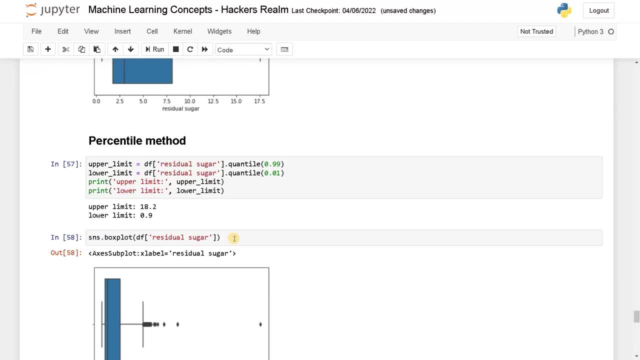 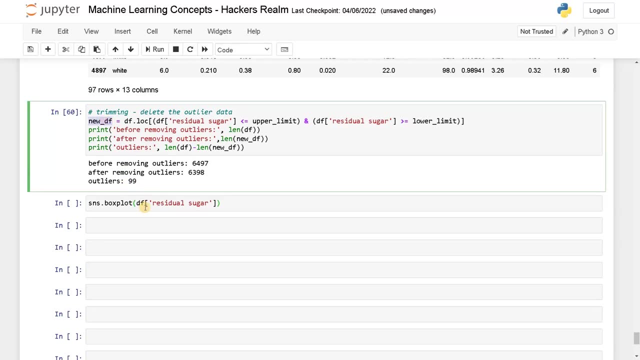 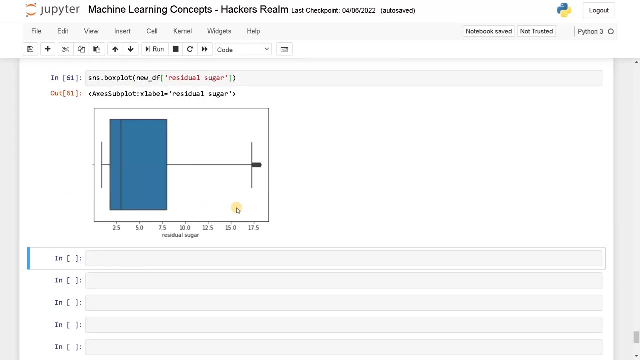 Now let's do the exploration again. So this will be new df. So again, you can see from this representation it changed to this. So we have removed data that are less than 1% And more than 99%. So this is trimming. 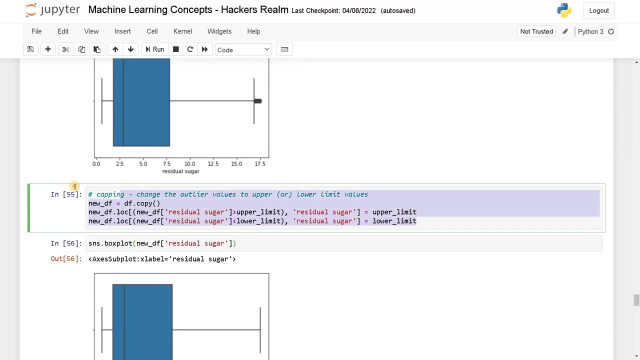 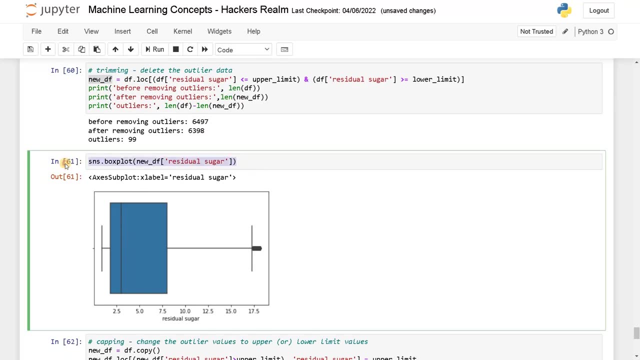 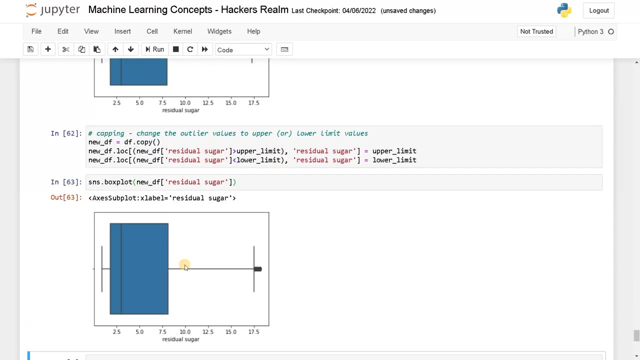 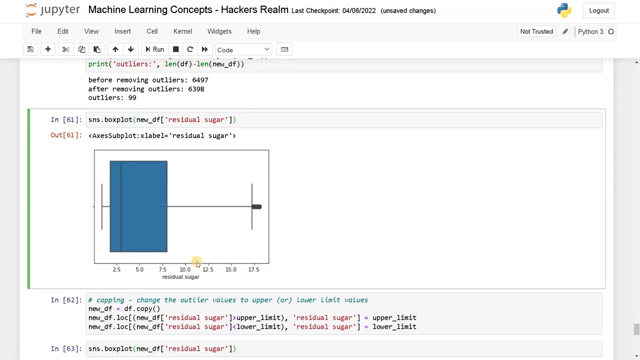 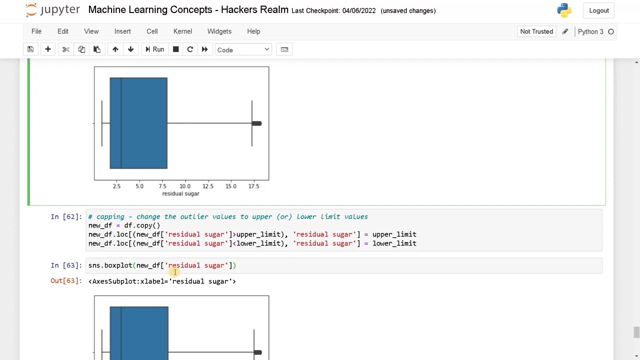 Now let's do the capping. let's again display this. As you can able to see, it's giving us a similar representation as trimming, without losing the data. So this is it, guys. These are the various method you can use in order to detect and remove the outlayers. 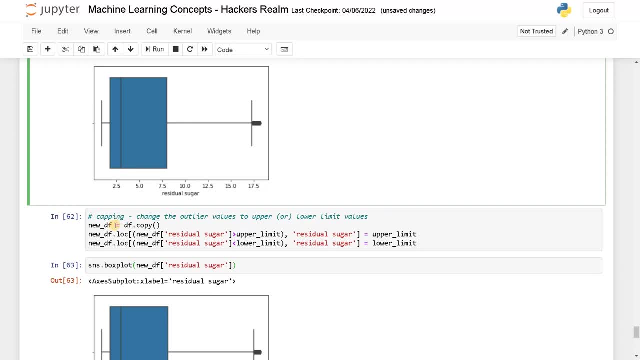 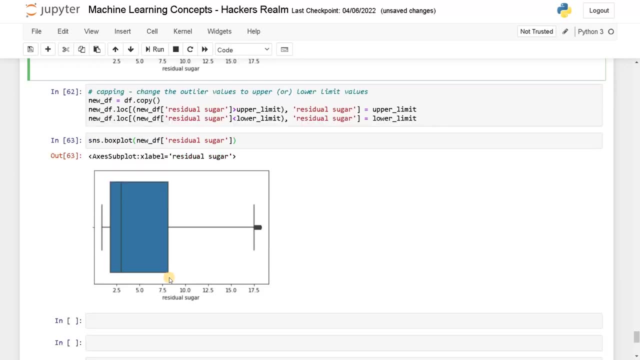 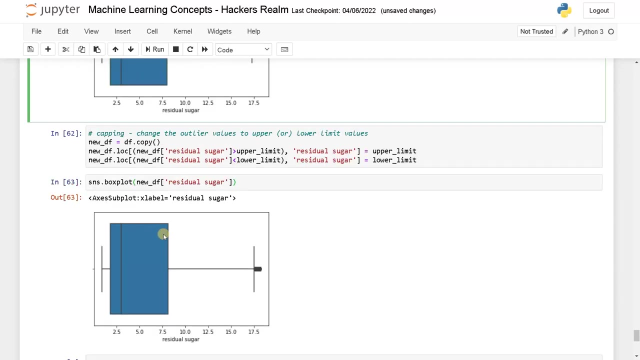 So I suggest you go for capping method, because it didn't remove the values, but it will change those values in that particular column. But it will give you a good representation of data and it will also remove the outlayers. Let's also display that graph with display. 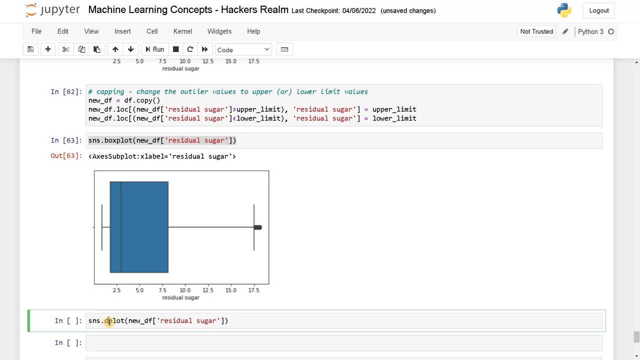 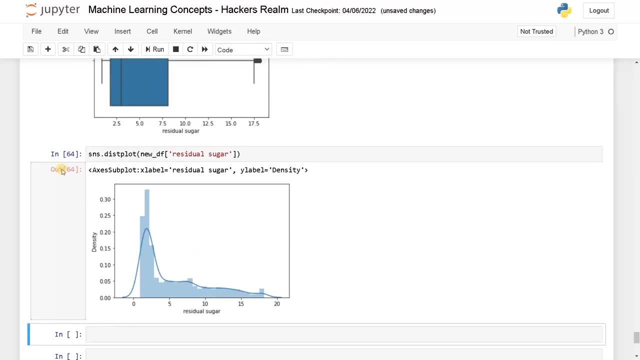 So this is it, guys. So this is the graph with this plot to see how it looks. Now you can see all the skewed distribution has been removed. Maybe for the comparison, I will also use the original data. So this is the original data and after removing all these outlayers, the data looks much more. 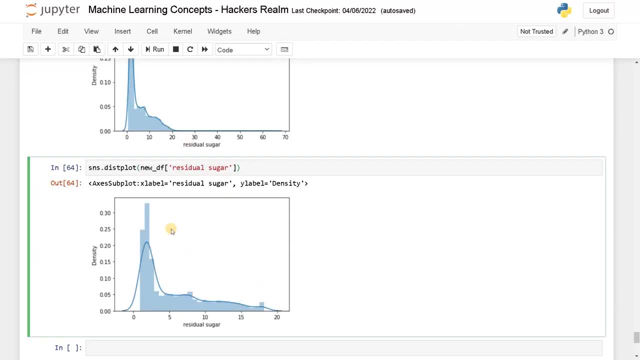 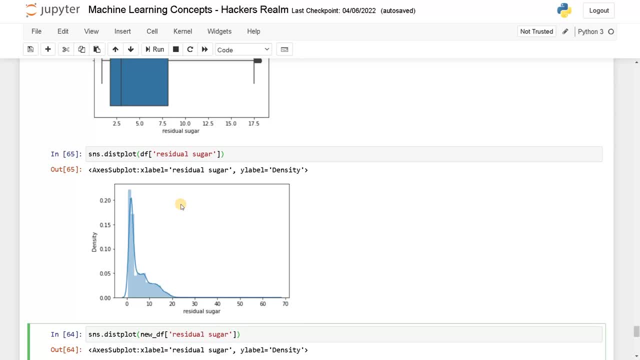 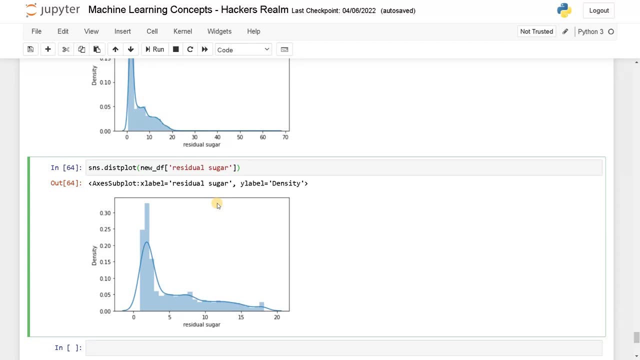 So you can use these two plots in order to detect the outlayers and transform the data in order to get good results or improve the model performance. And that's pretty much it, guys. In this video we have seen three methods: z-score method, interquartile range method. 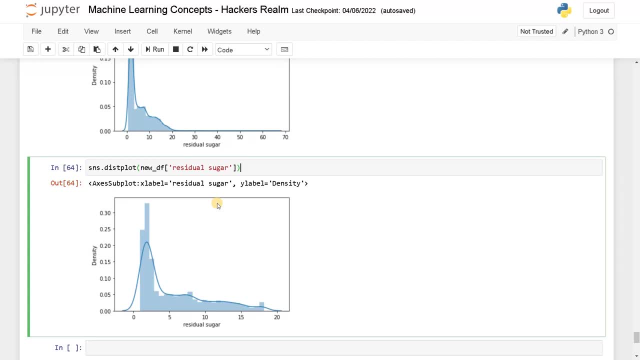 and lastly, we have seen the percentile method. If you have any queries around these topics, please leave a comment below. Apart from that, if you like the video, hit the like button and don't forget to subscribe the channel for more videos. Stay tuned for the next video. 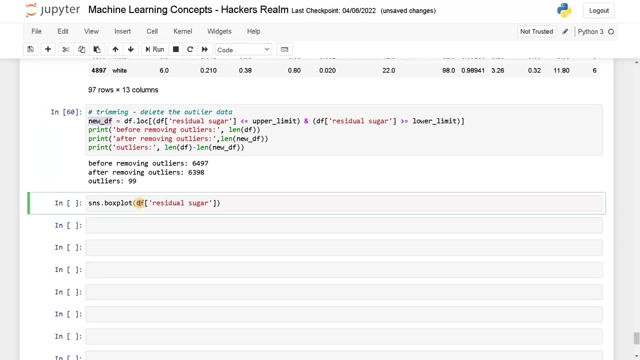 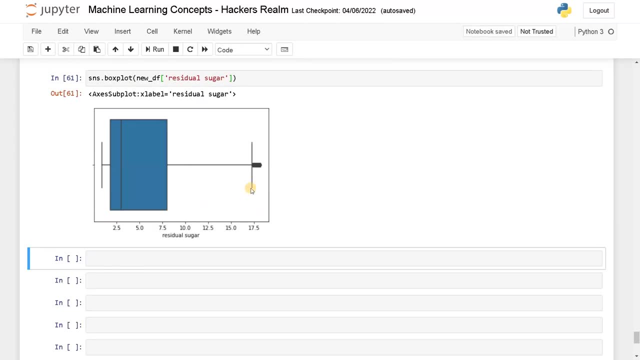 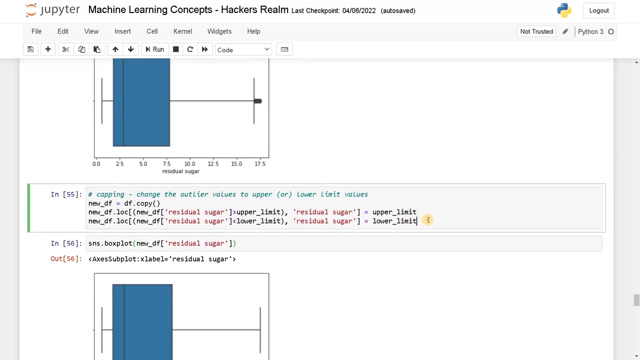 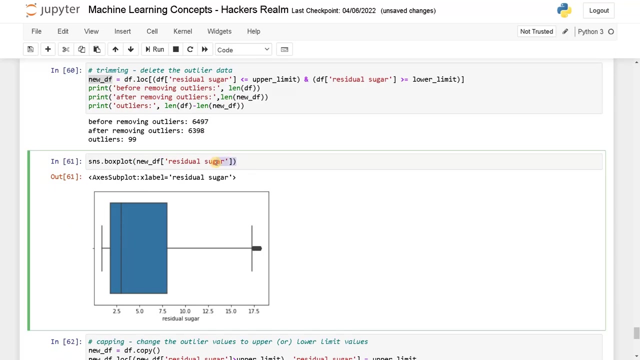 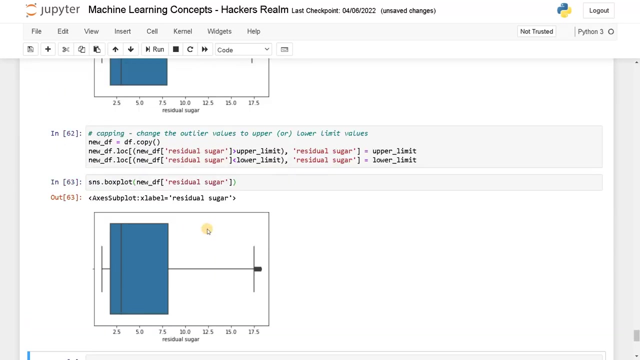 so this will be new DF. so again, you can see from this representation it changed to this, so we have removed data that are less than 1% and more than 99%. so this is trimming. now let's do the capping. let's again display this as you can able to see. it's giving us a similar. 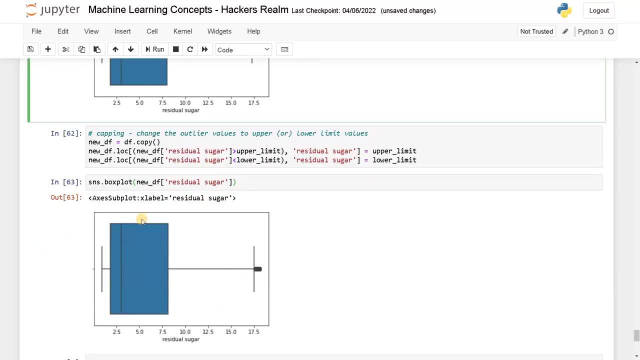 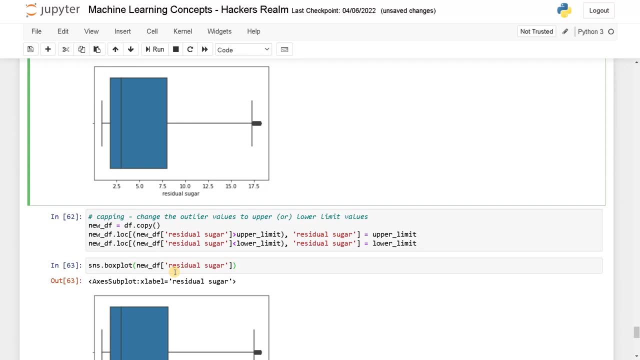 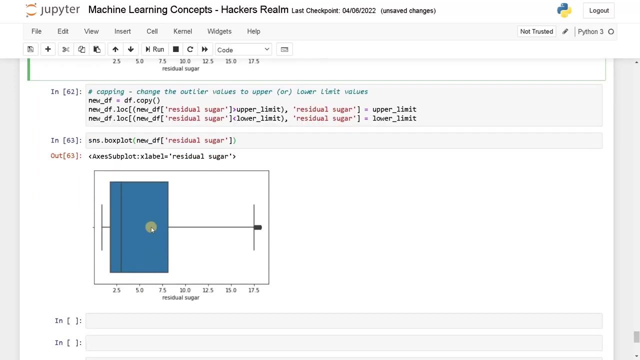 representation as trimming without losing the data. so this is it, guys. these are the various method you can use in order to detect and remove the outliers. so I suggest you go for capping method, because it didn't remove the values, but it will change those values in that particular column. but it will give you a good 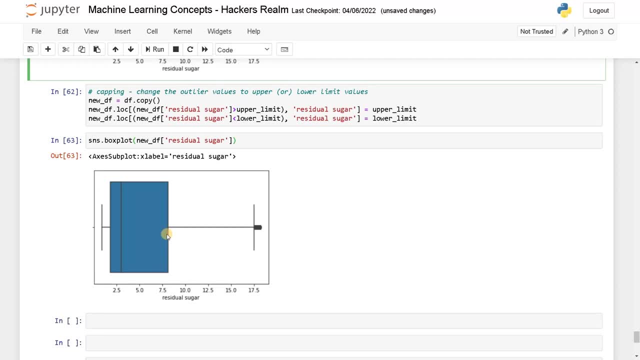 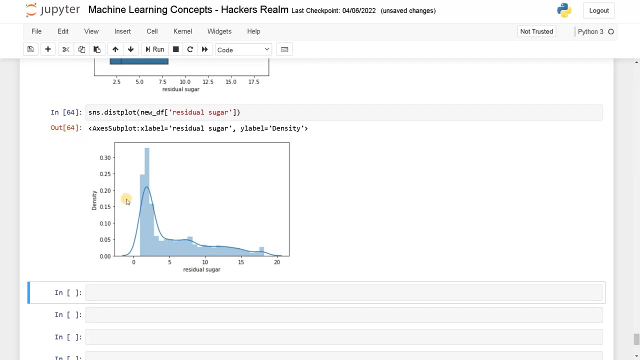 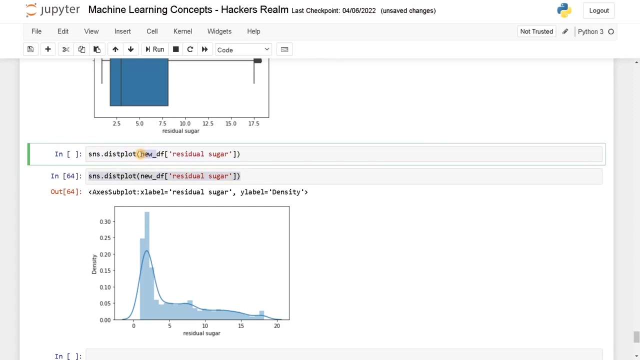 representation of data and it will also remove the outliers. let's also display that graph with this plot to see how it looks. now you can see all the skewed distribution has been removed. maybe for the comparison I will also use the original data. so this is the original data and, after removing all these outliers, the data. 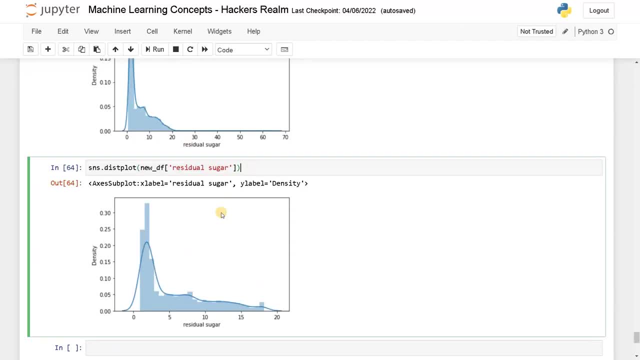 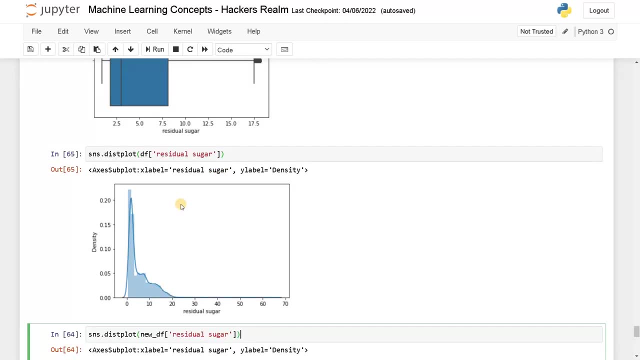 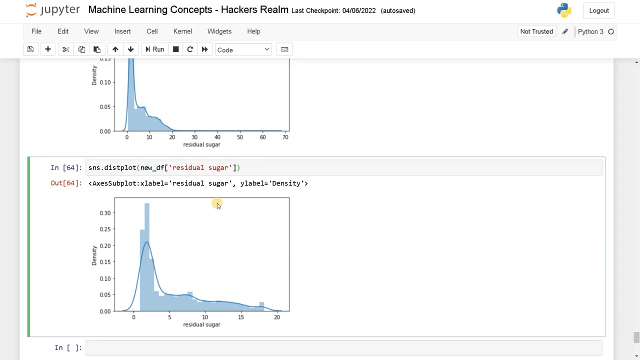 looks much more better. so the distribution looks much more better in the dis plot. so you can use these two plots in order to detect outliers and transform the data in order to get good results or improve the model performance. and that's pretty much it, guys. in this video we have seen now three methods: the 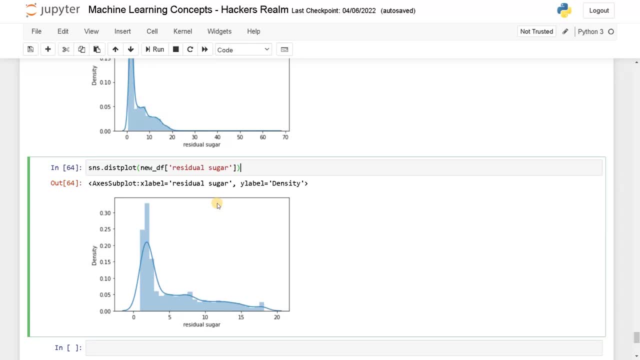 z-score method, interquartile range method and, lastly, we have seen a, the percentile method. if you have any queries around these topics, please leave a comment below. apart from that, if you like the video, hit the like button and don't forget to subscribe the. channel for more videos. stay tuned for the next video.